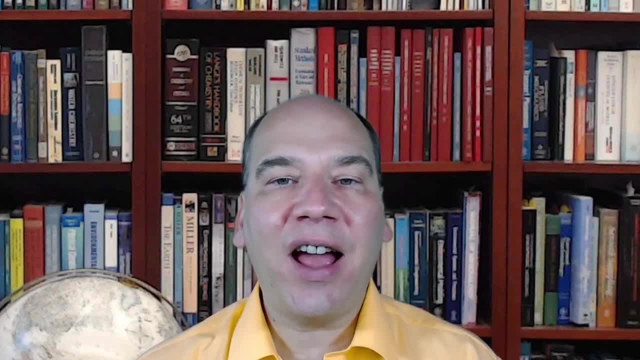 an hour later and one of the blocks is now warmer 100 degrees Celsius and the other block is now colder, zero degrees Celsius. And I didn't have any kind of external heat interaction with the block. I didn't have a thermal agency, no type of action. I just say to you that was spontaneous. 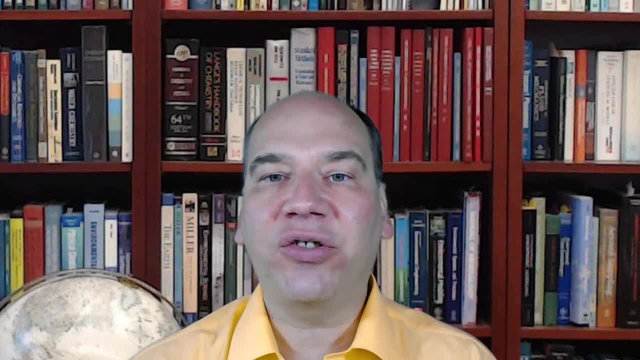 Well, I did conserve joules. I didn't create or destroy any joules. So I'm okay on kind of conservation of energy, internal energy, first law of thermodynamics. So something's missing that is not captured by that perspective And you say, well, yeah, that just doesn't happen. 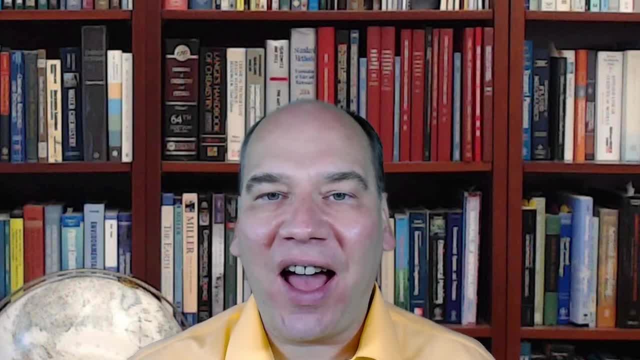 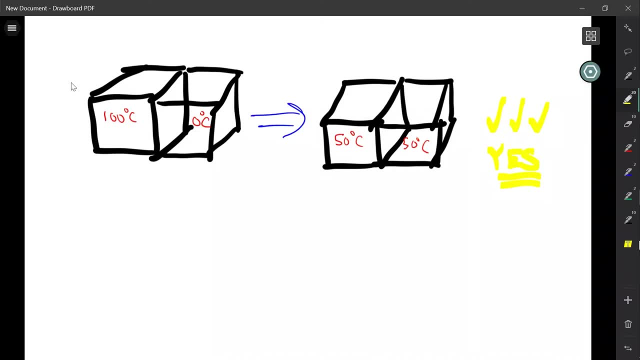 It's not the way the world works. When two things of unequal temperature in contact, the warmer one gets colder and the colder one gets hot. That's just the way it works. When two things are at the same temperature, they don't just spontaneously separate and 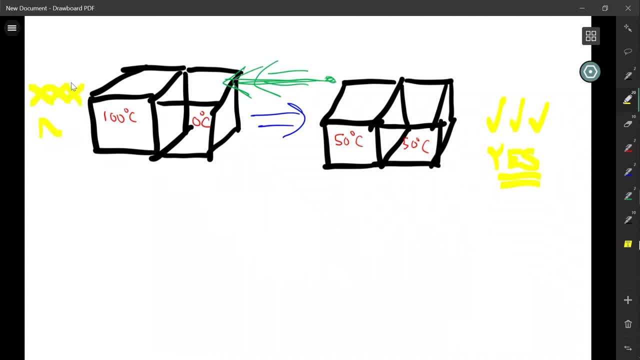 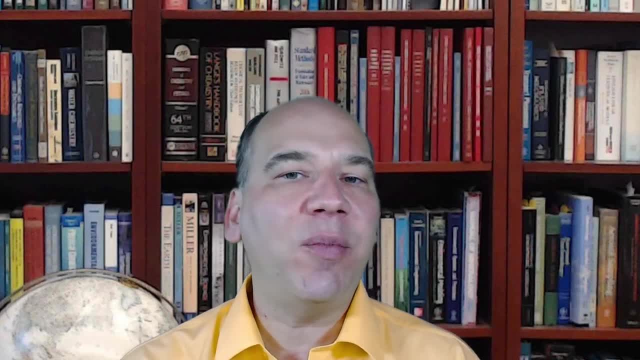 diverge in temperature so that one starts getting hot, one gets cold. It's not the way the world works. Well, you're right, We look around the world and that's not the way the world works. So we need something more. There is kind of, if you will, a directionality, an arrow of time. 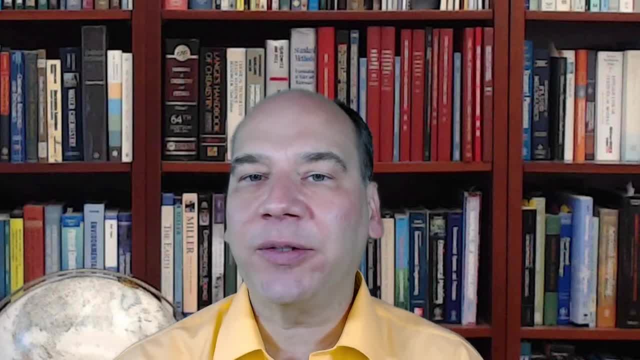 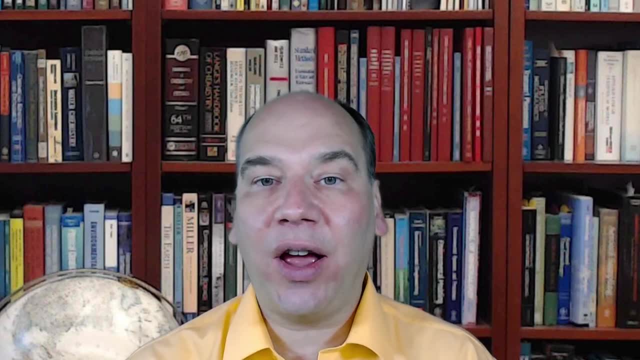 This is what's caught up in the second law of thermodynamics: that the direction of temperature is not the way the world works, So we need something more. The way we observe it is in one direction: Hot things cool, and then cool things get hot. 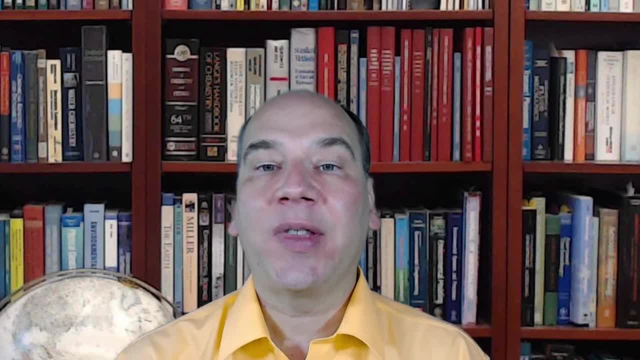 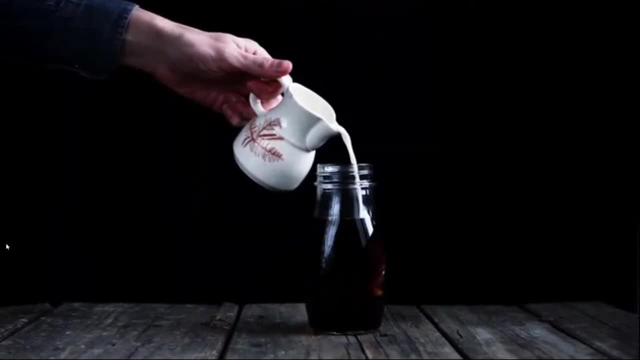 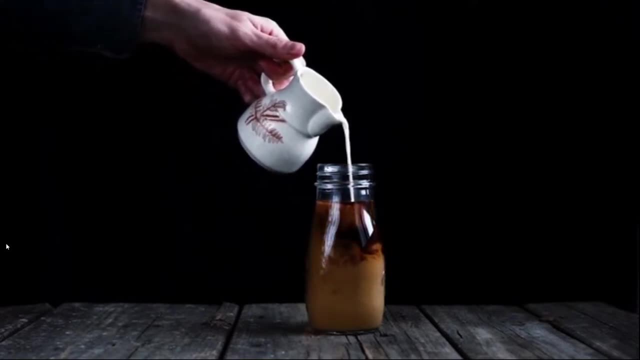 It's not the other way around. Let's take coffee and milk. If you start with some coffee and you pour in some milk and stir it around, you know they get mixed up with each other. That just happens, It's spontaneous. That's the direction, No matter how long you leave that mixed. 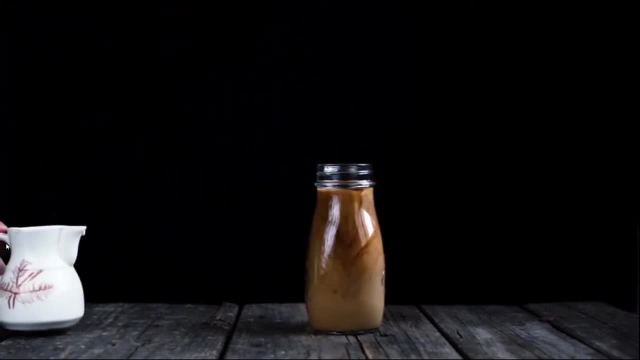 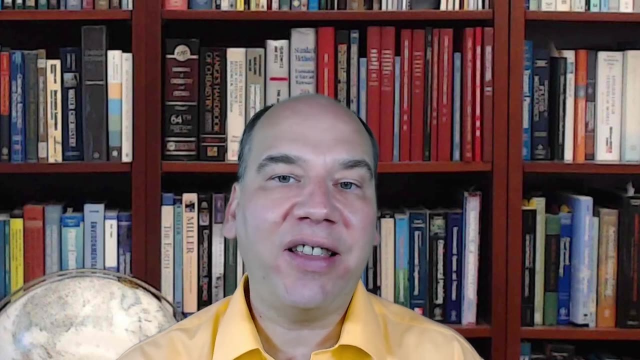 coffee and milk together. it doesn't separate back to pure milk and pure coffee. It just doesn't happen. That's not the way the world behaves Energetically. that could be okay, but there's something about a directionality of time, a spontaneous direction that things happen. 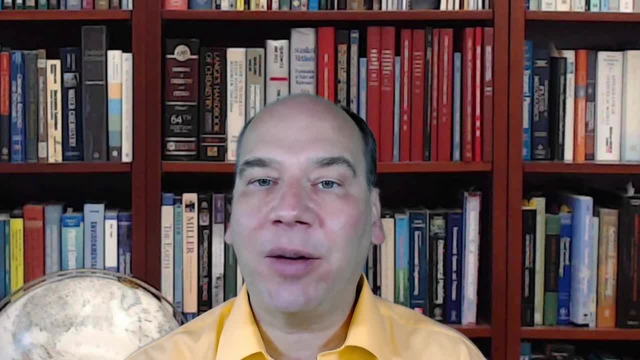 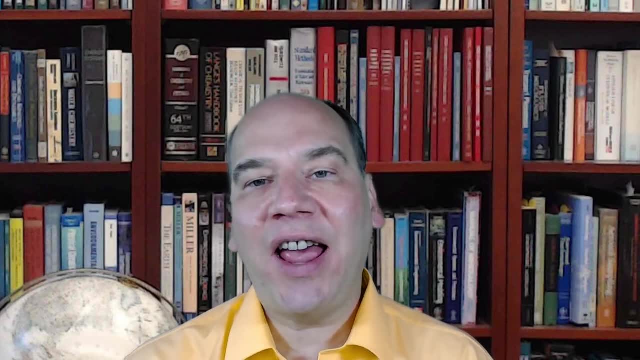 We need something more. Again, we need this second law of thermodynamics to help us explain the way the world behaves. Another example: we have a high, we have a tank of high pressure compressed gas. Maybe at home you've got a CO2 infuser to make your own sparkling water. 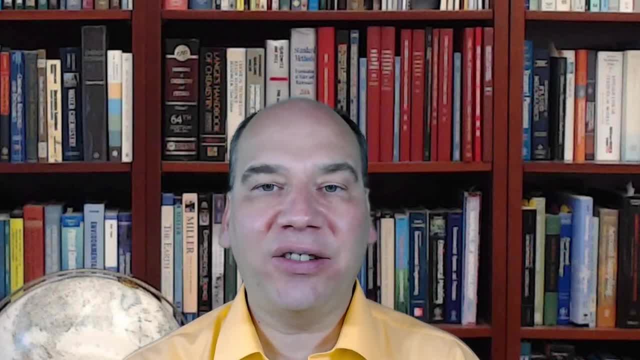 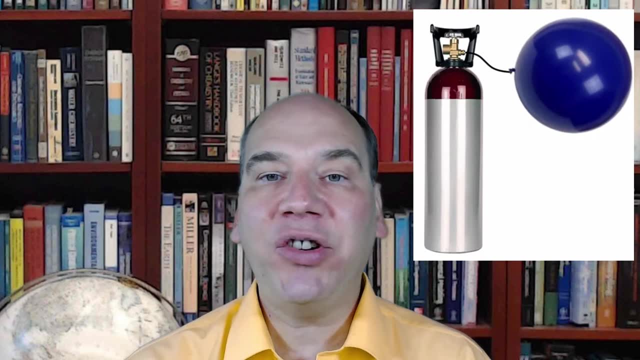 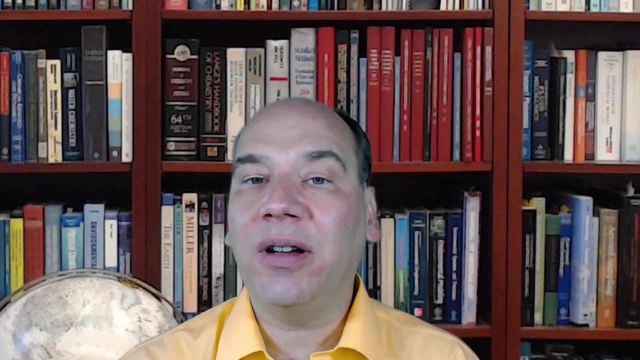 or maybe you've got access to a nitrogen tank to blow up some balloons. But we know that if you open up that valve, the high pressure gas goes out in the atmosphere. It just happens that way. No matter how long you wait, those temperatures are equalizing. High pressure wants to go to low pressure and, in consequence, low pressure starts to increase to meet the high pressure and at some point you have an equalized normal pressure. No matter how long you wait, you're not just going to have an equalized normal pressure. 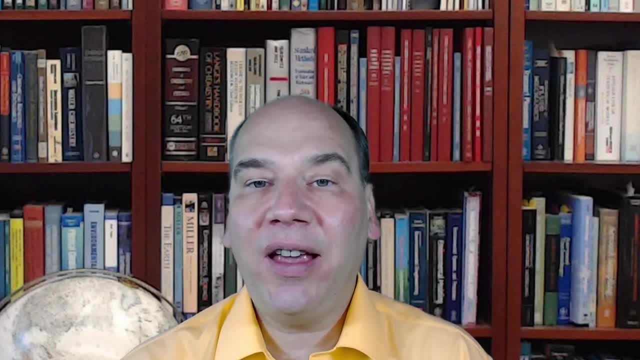 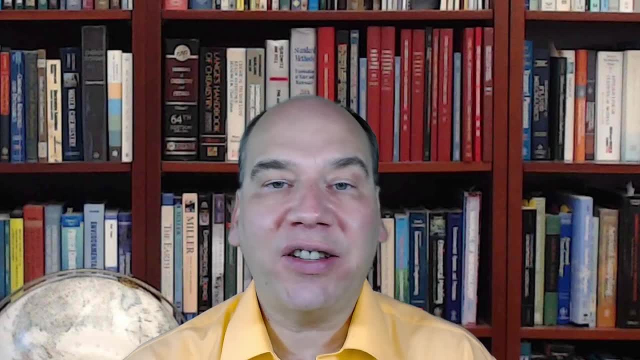 that suddenly the gas accumulates again in the cylinder all on its own and leaves a vacuum outside or a lower pressure. That's not the direction that things work. So we need something more, and that's the second law of thermodynamics that talks about the spontaneity of the direction. 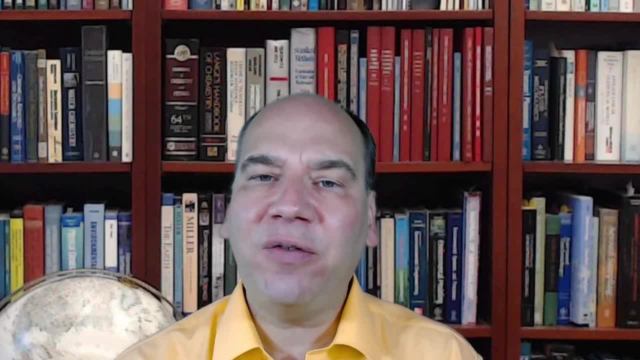 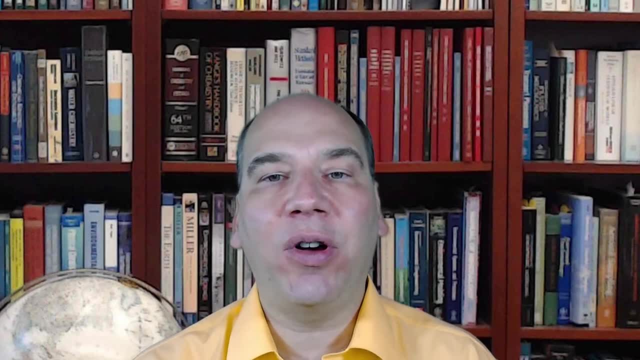 of change And that the way we've discussed it so far is qualitative. If we want to quantify it. that's where we're going to introduce the mathematics that we'll call entropy. We're going to introduce a quantity called entropy. It'll be given the symbol S. We'll 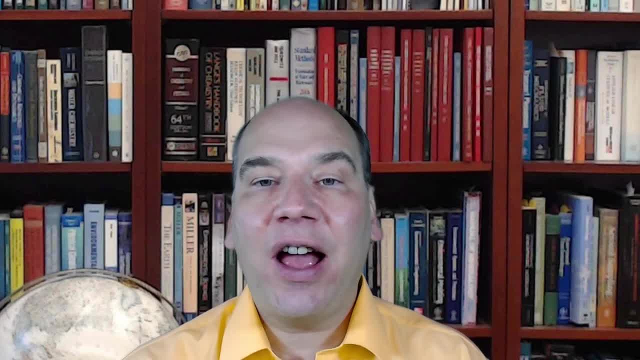 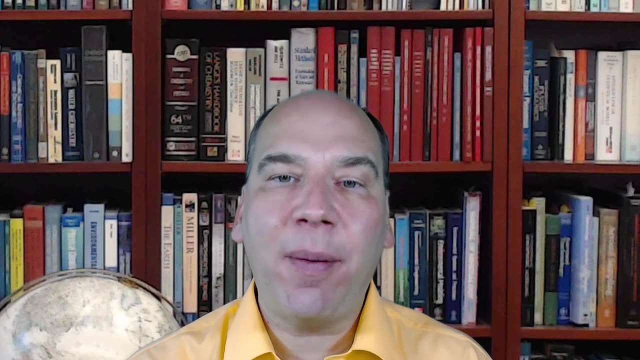 get into that. But that allows us to actually quantify this idea of non-spontaneity and spontaneity. How spontaneous was it? How non-spontaneous was a proposal? We want to put a number on it and that's going to be this symbol S for entropy, which we'll get. 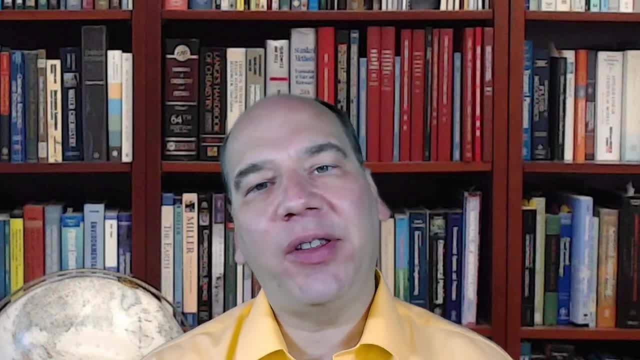 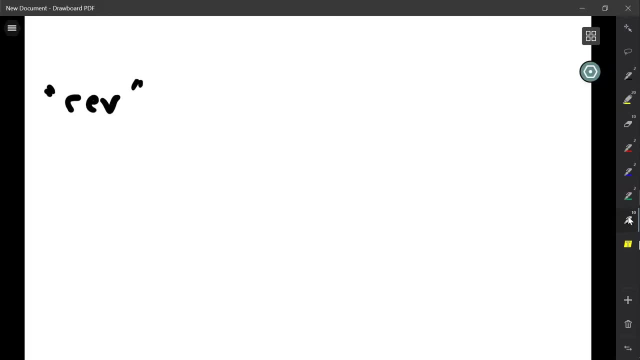 into. Okay, a critical concept to think about or introduce are what we're going to call reversible or irreversible pathways. As we go from an initial state to a final state, are we following what's called a reversible pathway or are we following what's called an irreversible pathway? This 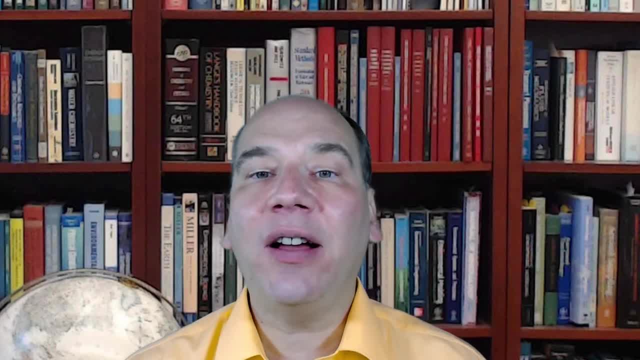 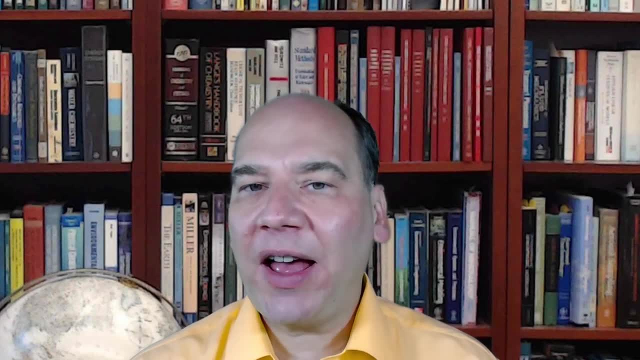 differentiation, or this concept can take a while to get used to. but it's going to take a while to get used to. So let me look at it from different perspectives. A reversible pathway means as you are moving along the path, at any point you can stop and go backwards. So, for example, if we are 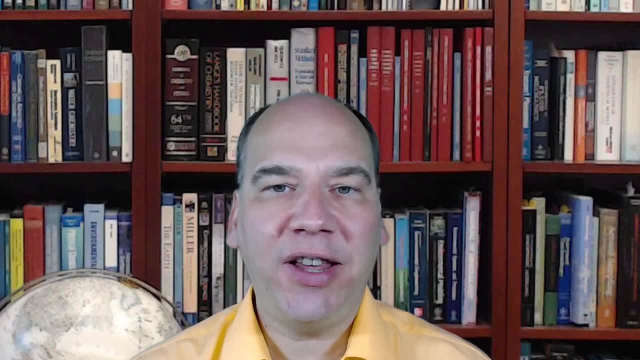 raising a weight on a frictionless pulley. we can pull that weight up and we can interrupt it at any point and go backwards with non-spontaneity. So, for example, if we are raising a weight on a frictionless pulley, we can pull that weight up and we can interrupt it at any point and go backwards. 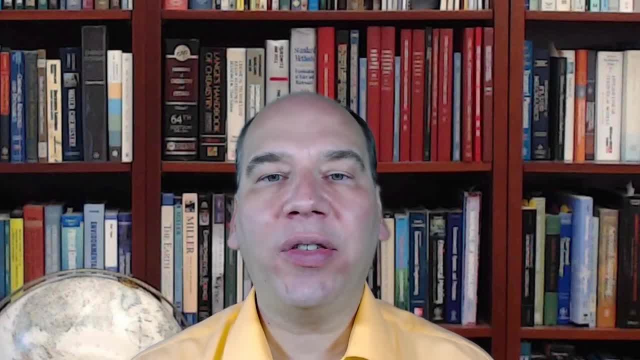 Let's contrast that with having something that is at high pressure- a gas- and then opening the valve and using that to push back the atmosphere. Well, that pressure comes rushing out and at no point can you just stop it, that rushing out pressure. 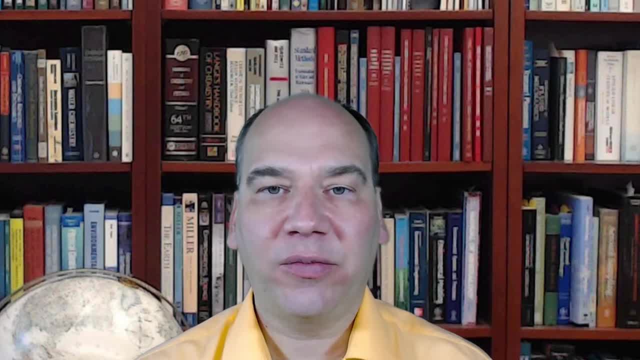 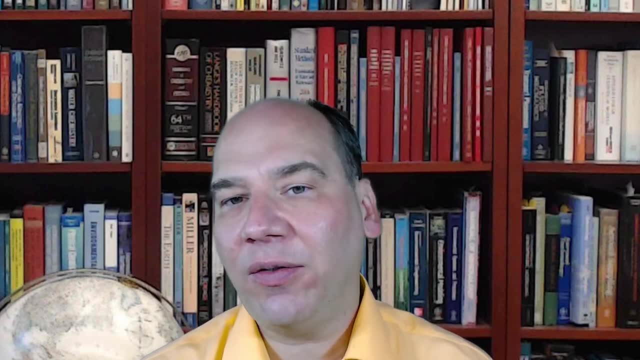 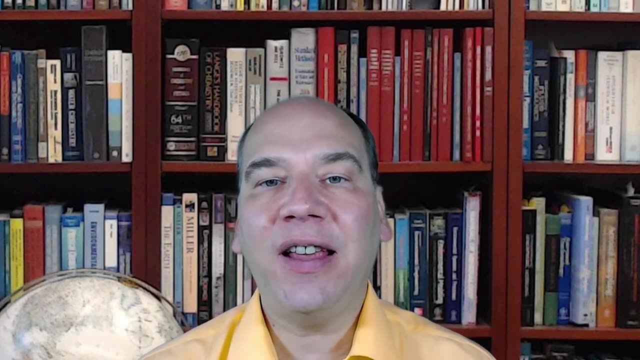 And just have it go backwards and call that irreversible. What are some of the characteristics of trying to define between a reversible or an irreversible? Well, let's take some of these state variables like temperature pressure. If it is irreversible, you can't really sometimes say what they are along the 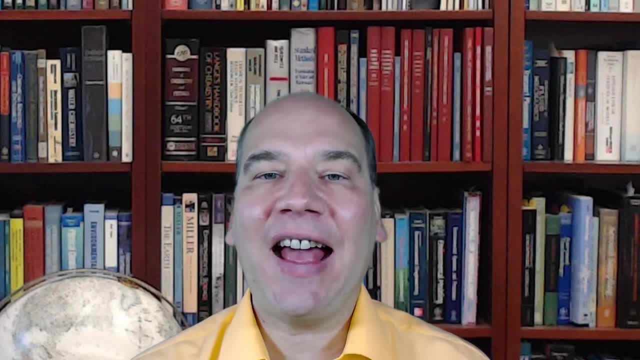 path. So example: this strongly expanding gas from a cylinder into a low pressure region. Well, you have wave fronts of that gas coming out. It's going to have a lot of heterogeneity. You know, you can't really say what the pressure is during that time period because they're little pockets of gas. Some of it are probably 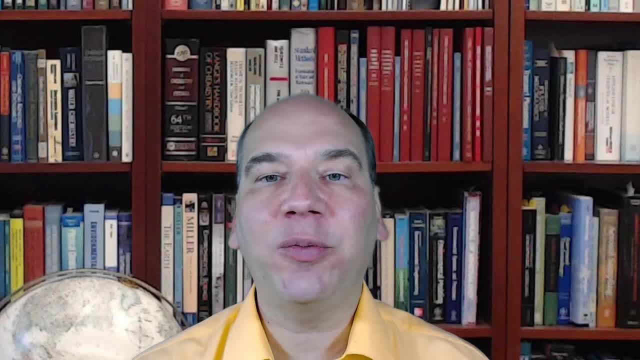 what you might call more local concentrations of molecules per cubic meter, some at higher, some heterogeneity of pressure. You don't really have a pressure statistic. that bolus of gas, It's just a bit chaotic coming out. Similarly, if we have 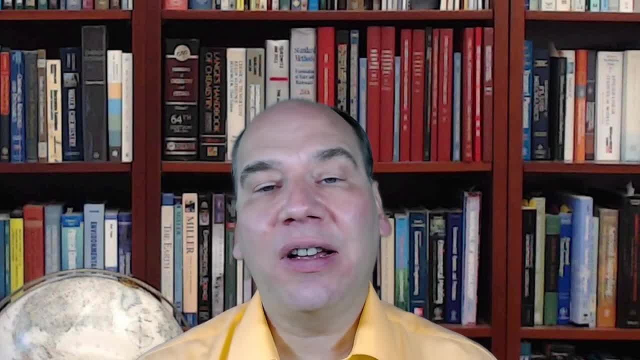 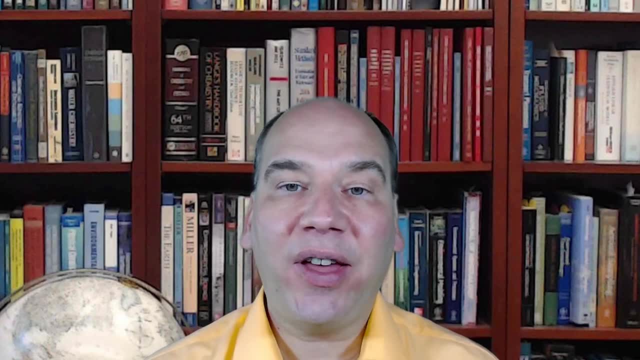 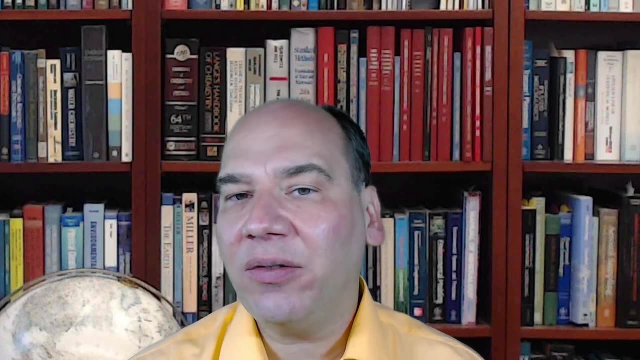 something at a high temperature, that is, transferring joules to something at a lower temperature, say 100 Celsius in contact with a 90 Celsius. During that heat transfer you don't really know what the temperature is in the intermediate regime. Depending on the nature of the heat transfer, you might have variabilities in joule. 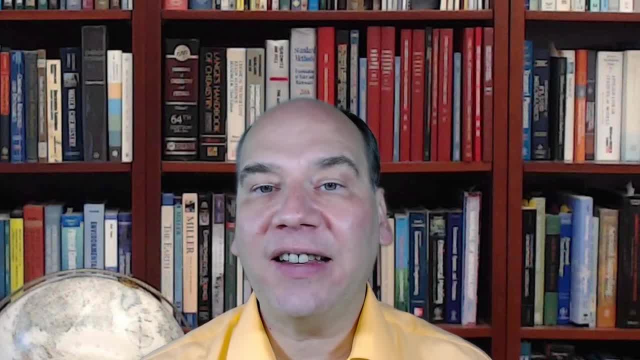 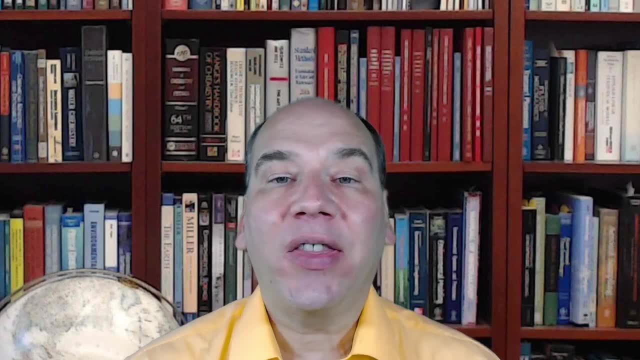 transfer rates where the two materials are better connected. where they're not as well connected, They can change the temperature of the gas. You don't really know what the temperature is across that temperature jump. So again, that's another characteristic of irreversible. 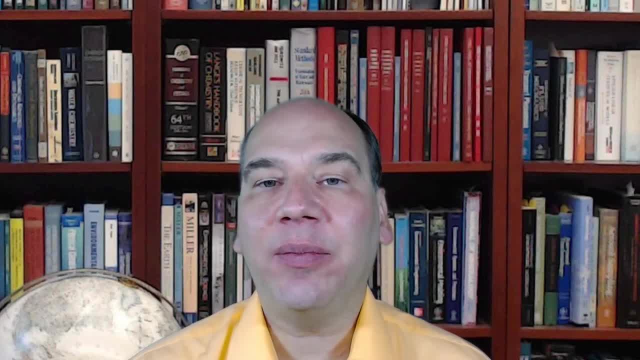 In point of fact, reversible processes. anytime you have a real process, a reversible process, well, if you don't have any friction, then it's going to take you forever, an infinite amount of time. So, if you don't have any friction, then it's. 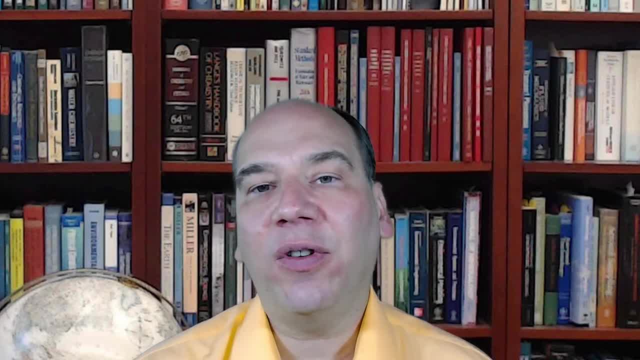 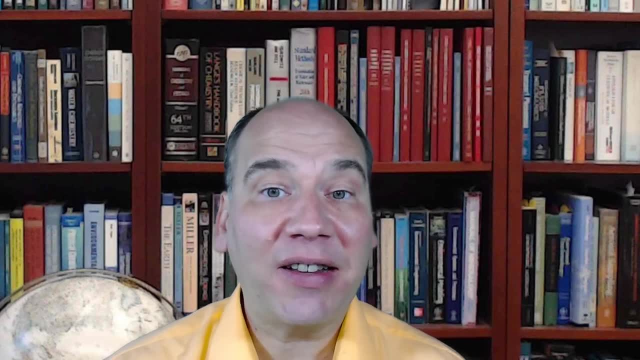 going to take you forever, an infinite amount of time. So if you don't have any friction, then it's going to take you forever, an infinite amount of time. So a reversible process is also something that typically takes an infinite amount of time to take place. If you're going to be pushing back a cylinder, doing some. 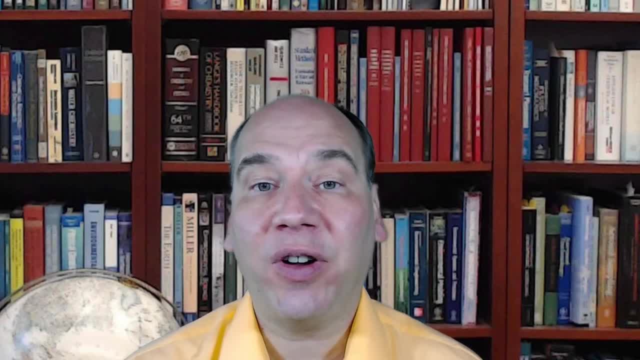 kind of pressure volume work, pushing back a cylinder. if you want to avoid friction and you want to know what the pressure is at every point and you want to know what the volume is at every point, well, you have to do that infinitely slowly in order to get a. 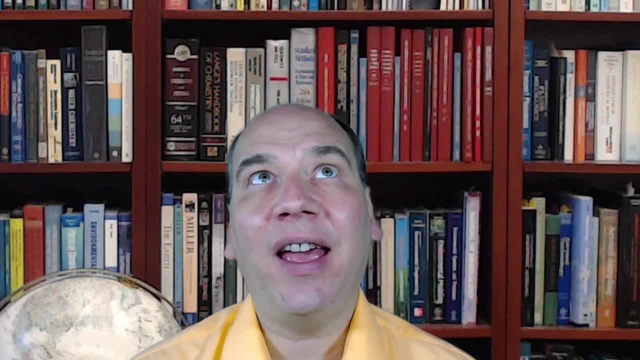 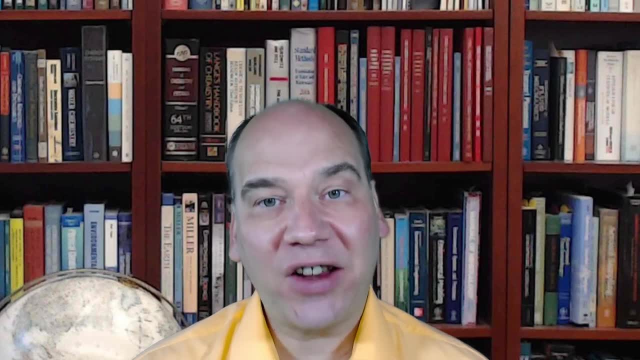 reversible process. So you might say, Well, well, okay, no, real processes are reversible processes, so why do we even talk about them? Well, and actually in thermodynamics, we often, always talk about reversible processes. And why is that? 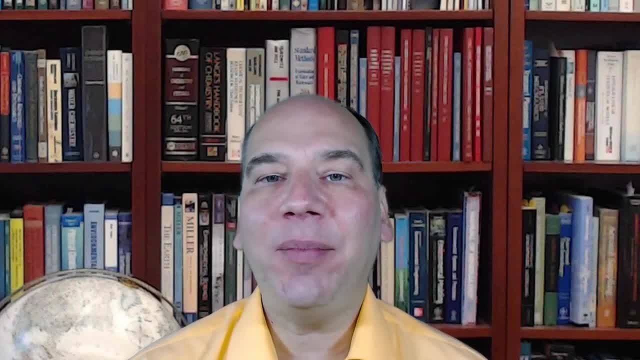 Well, because they're a limit, They represent a limiting behavior, say to efficiency of conversion to some energy source over to some desirable useful action. The thermodynamics represents an upper limit. The real world will be less efficient. I could go along. 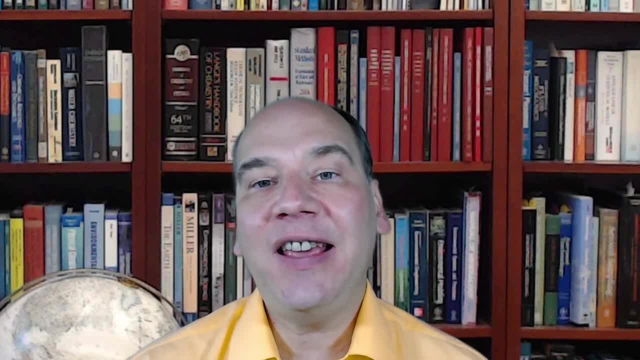 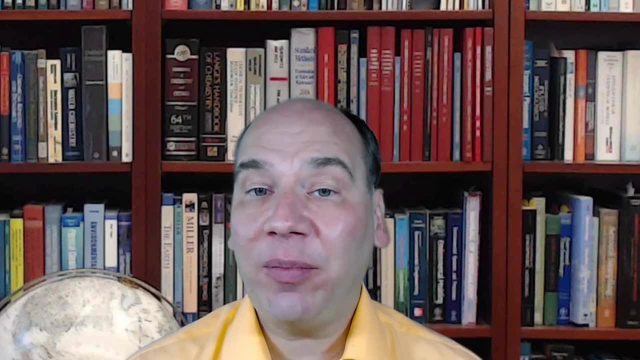 I could go along with a whole list of examples that way. But the reversible process, the one that is theoretical, the limiting process, often will take an infinite amount of time to actually do. Those are the best you can do and the limit Then we'll see in our definition, when we get to, of entropy, that thinking about the reversible pathway from an initial state to a fight. 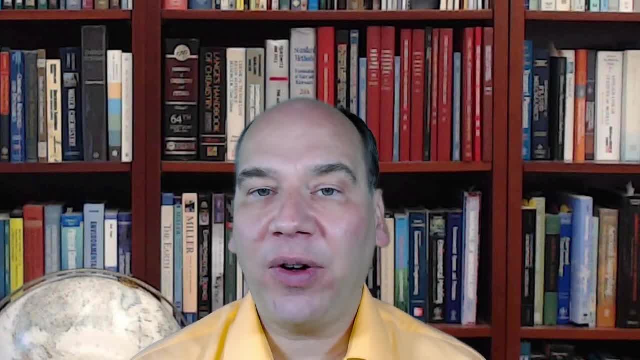 observation. If you then get to the right stay point and look at that, eventually you'll be looking at it at least for every cross, determine if it's real or if it isn't. Now, if we haven't done enough, Iím keeping the lately queued up for something interesting, especially with Geights: chocolates. 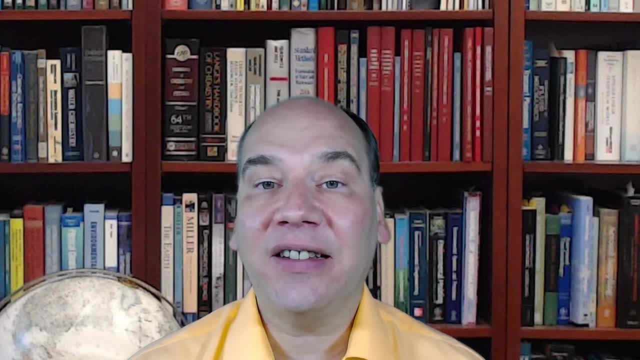 We went through a lot of things about it. I want to name countries, Just begun, as we go into it. Then we'll show you what you have need to do. Then we'll do final state. um, that is a a key thing that we're going to need, uh, to do. we're going to need to. 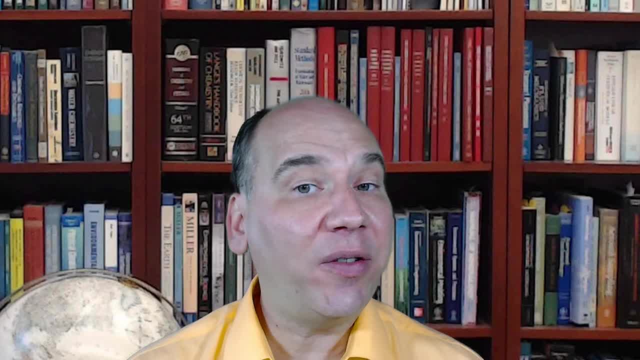 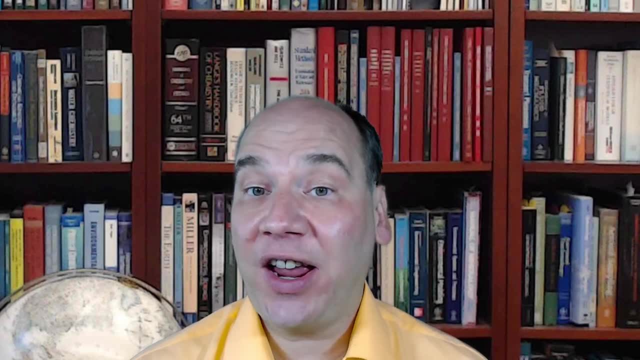 connect the initial state and final state by reversible, even if theoretical, by a reversible pathway in order to get at this quantity of of entropy change. and that then would be, uh, the entry change from the initial state and the final state, and even if it is the real pathway, is an 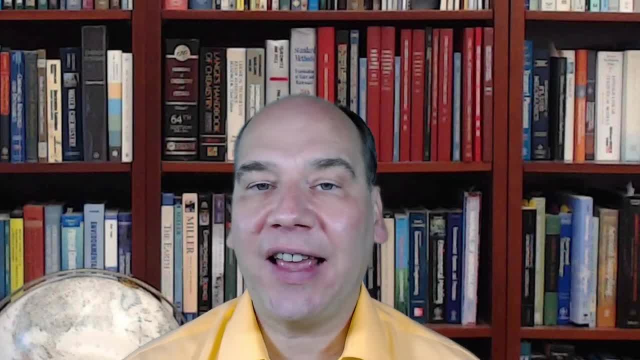 irreversible pathway, like a rapid expansion or something like that, the actual entropy change. entropy turns out to be a state variable, meaning it's independent of the pathway. so even though in the real world you follow an irreversible pathway, you can calculate the entropy change following a reversible pathway. again, this is a subtle concept that will come. 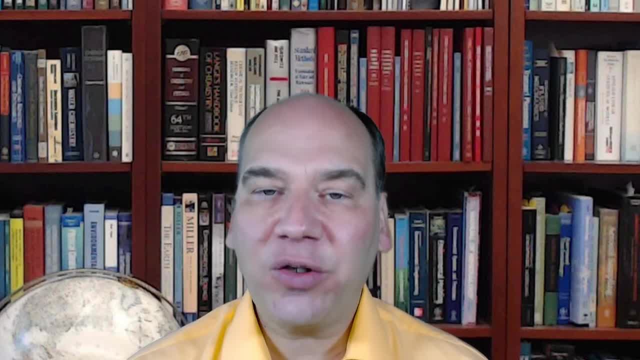 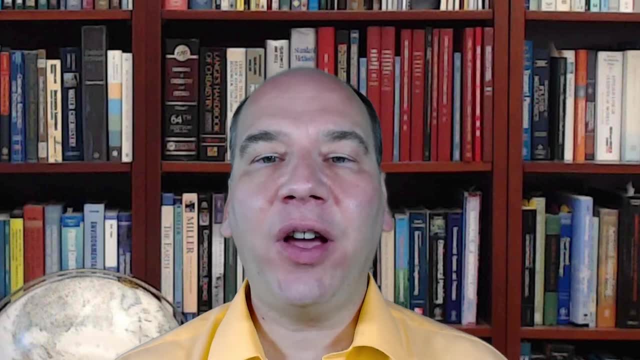 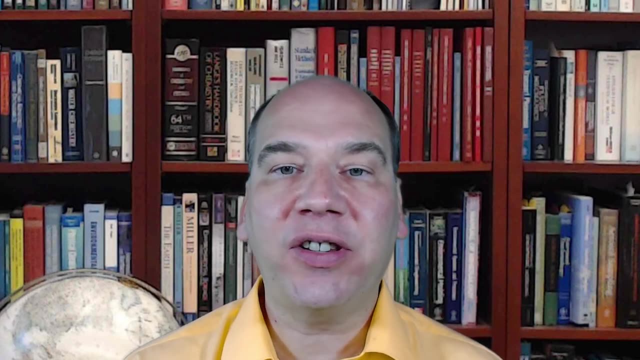 with practice. but to talk about entropy, we need to talk about reversible, which we just did. okay, let's give the equation. what is entropy? entropy is given the symbol s as you move along reversible pathway from an initial state to a final state. because it's reversible, you can do. 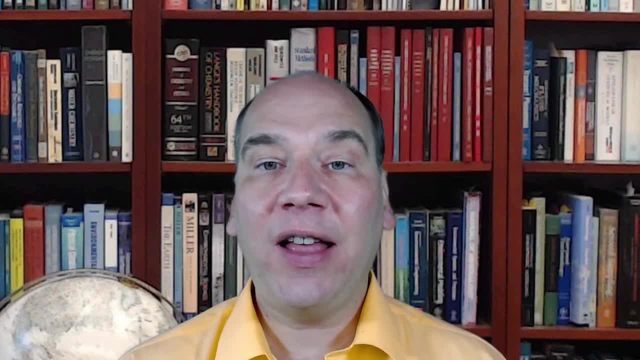 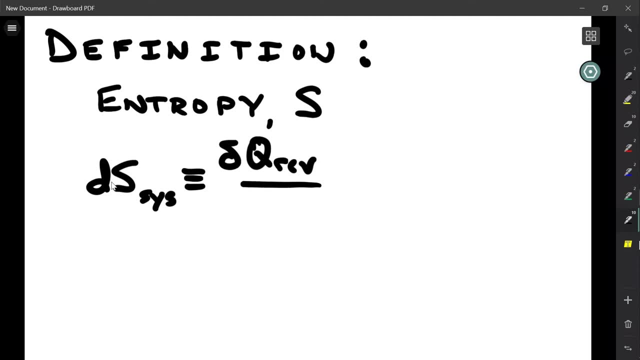 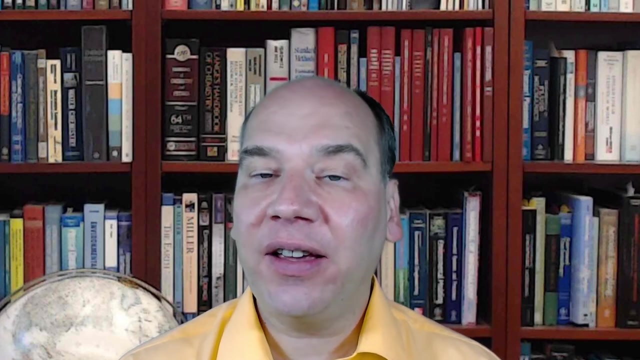 an incremental step, you can always stop and reverse it. well, at any incremental step, the entropy is defined. defined as ds equals the reversible heat interaction divided by temperature across that infinitesimal step. what i also want to say is that that definition is not unique, that we won't get into. 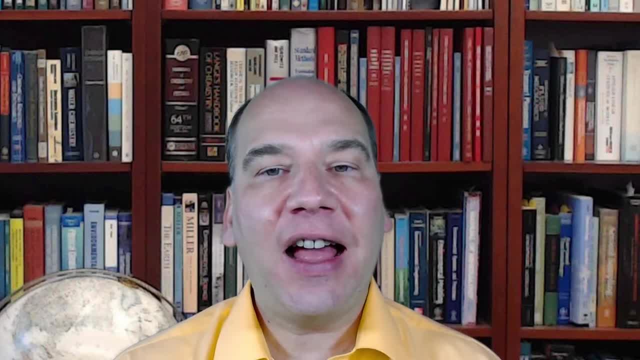 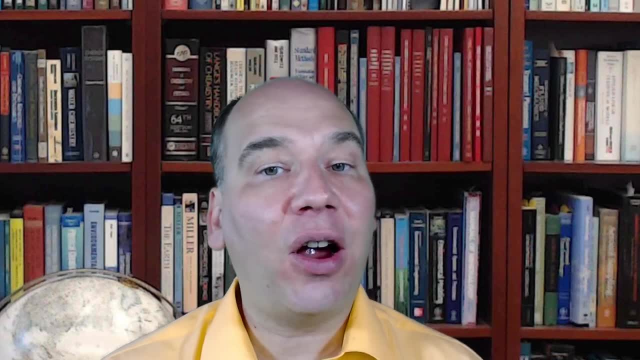 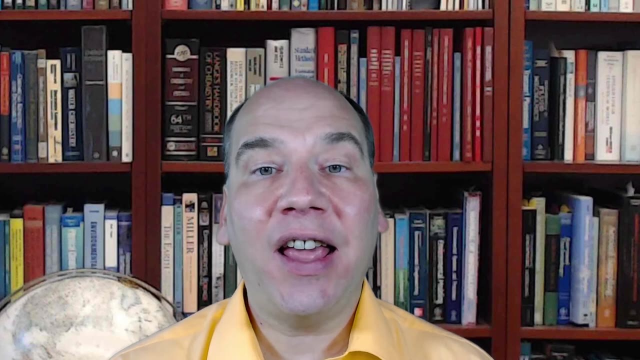 it. but just so you think that, just so you know that entropy is not something mystical or magical. it is simply a mathematical artifice that quantifies the change in reversible heat interaction, divided by temperature, across a pathway from initial final state. it's not unique, we could have used other. 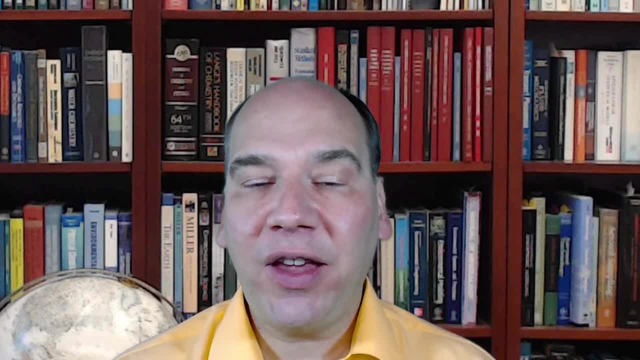 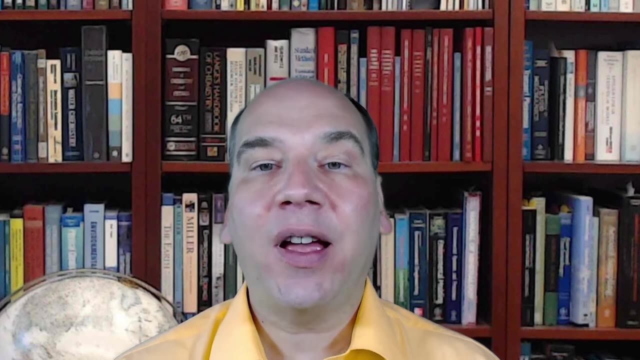 math and other math has been, uh, defined over the years. but it turns out, as we'll show, for example, that kind of a minimalist or simplest math to use is the definition that i just gave and it's the one then that is actually used most widely. but whether you use that one or another definition, 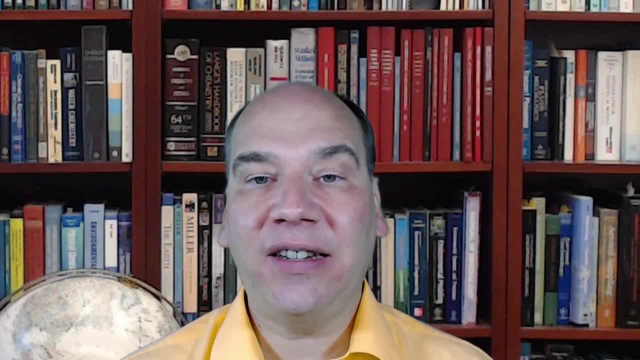 of entropy. all of that math is the definition of entropy and it's a very simple definition of entropy. you have to be self-consistent in the way you treat the universe. you have to define a mathematical function, entropy. i gave you one, but they're actually an infinite number. 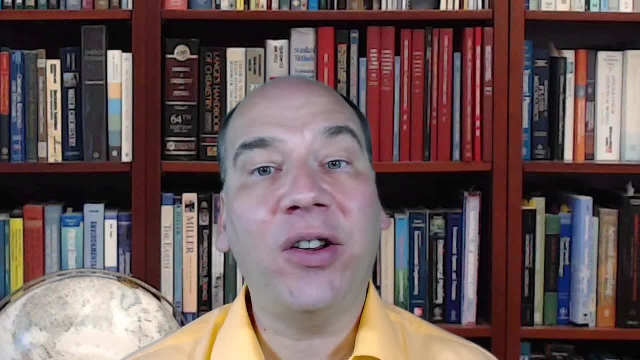 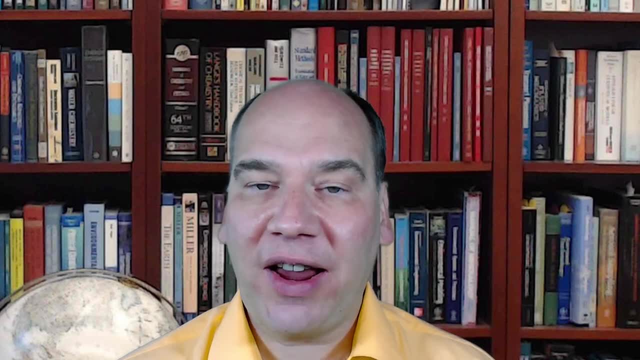 you can define if you get into advanced thermodynamics. i only say that to get emphasize that entropy is not a physical quantity. entropy is a state variable, which is great, and it's a state variable that allows us to quantify, um, what we know about the uh direction of time or the 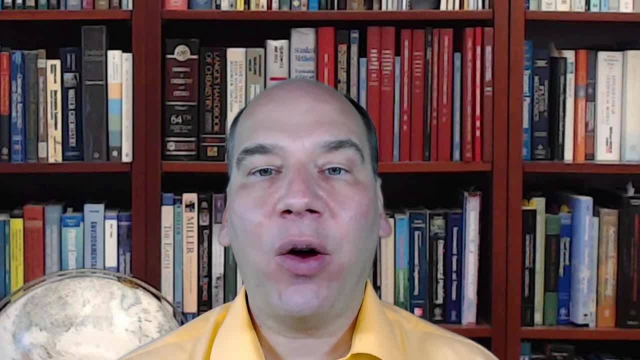 or the way that things work, that things next to each other- one cools, one warms- not that two things at the same temperature spontaneously separate temperatures to one being warm and one being cool. so entropy is simply a mathematical function that's going to allow us to track that and 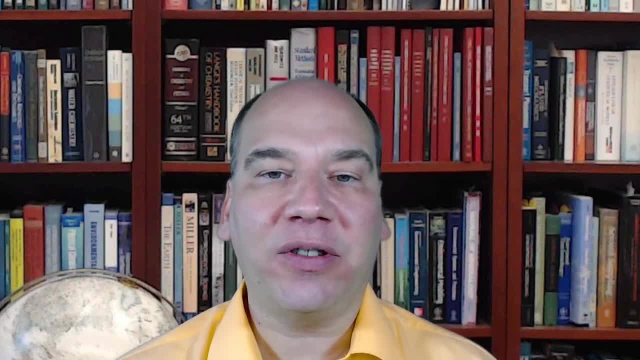 quantify it and keep track of it, almost like an accountant keeps track of it. entropy is not something we can measure, but it is something we can keep track of and it's very, uh, powerful. so at the end of the day, we're going to say that the total entropy of the universe- 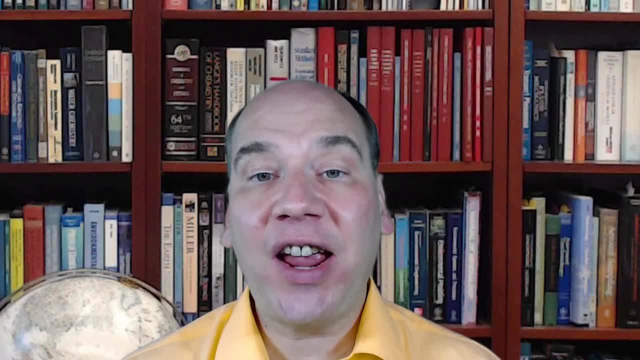 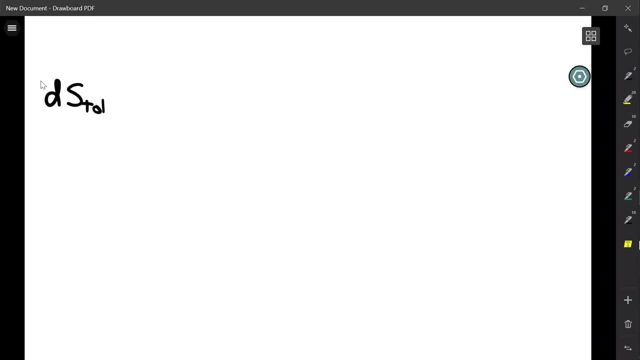 must be equal to or greater than zero must change. the change in total entropy of the universe must be equal to or greater than zero for any process we consider. so, to unpack that a little bit, if the total change in the entropy of the universe is zero, it's a reversible process. 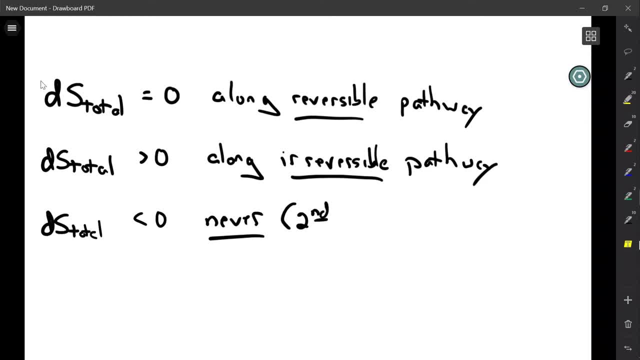 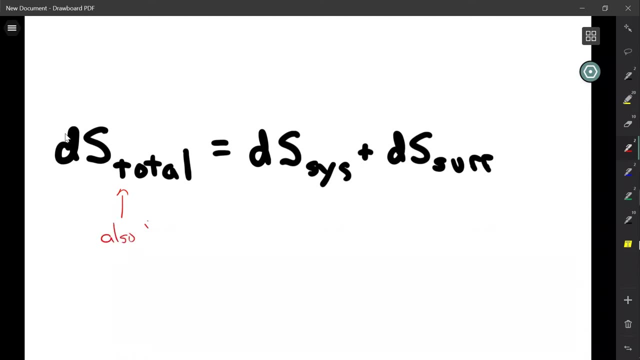 if the total change and entropy the universe is greater than zero, then it is, uh, an irreversible process. and i said their total entropy. this is quite important because most of the other things we've spoken about we've really just focused on the system temperature: temperature of the system. 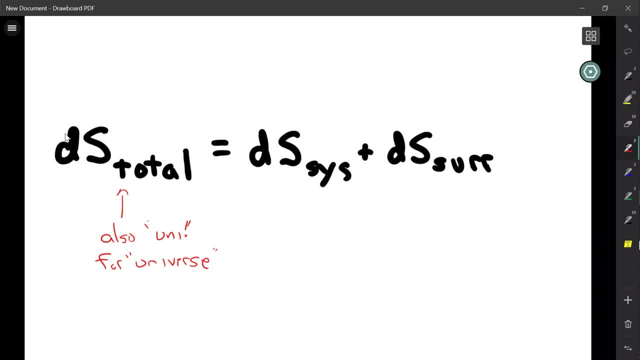 pressure: pressure of the system. volume, volume of the system. internal energy: internal energy of the system. kinetic energy. kinetic energy: the system. we've often been able to ignore the surroundings. well, when we talk about entropy, you always have to be very careful, because sometimes we could be talking about. 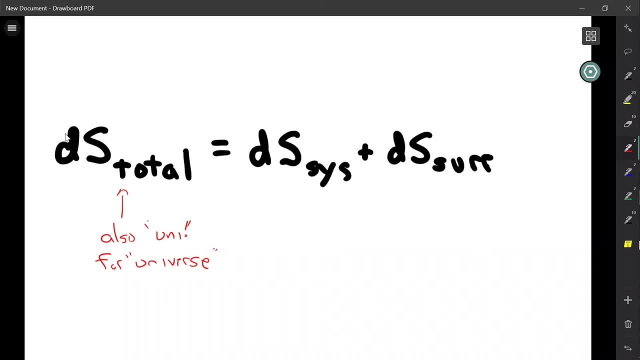 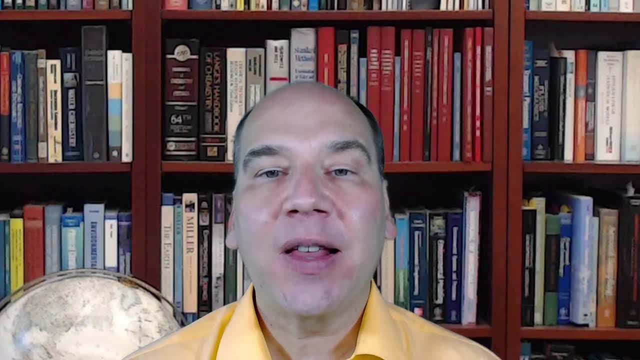 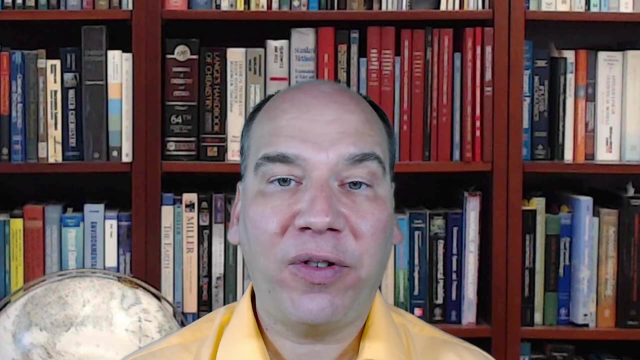 entropy of the surroundings. sometimes we could be talking about entropy of the system. sometimes we could be talking about the two of those being added together, which is the total entropy, and occasionally we'll get a little sloppy and we'll leave, say, the system subscript off of entropy and 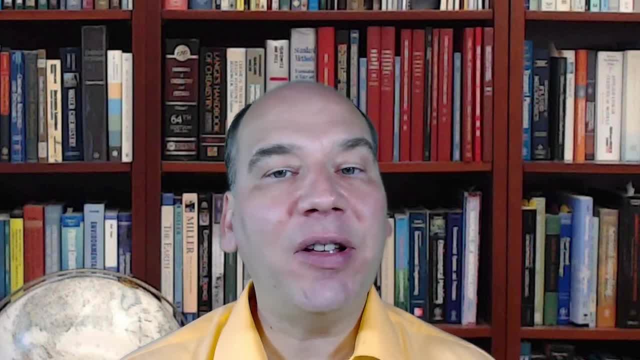 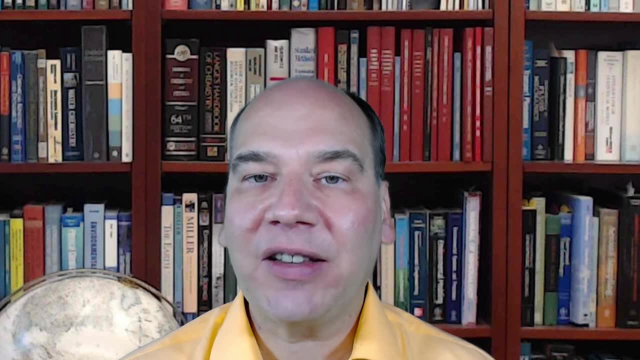 so you might think it's a total entropy, but in that case maybe it's only the system entropy, so you can be careful about these contextual tools. and then, like most of the other variables in thermodynamics, entropy stands out as a particularly vexing one, just in terms of labeling, and that we 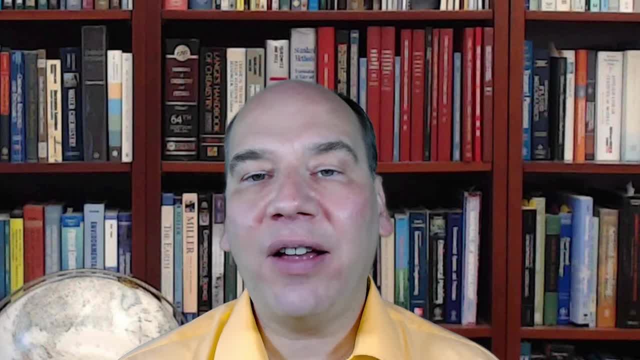 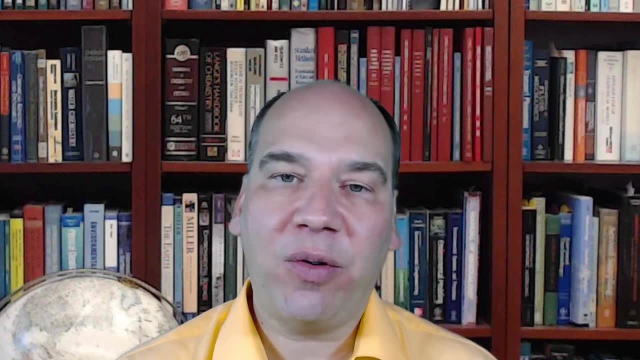 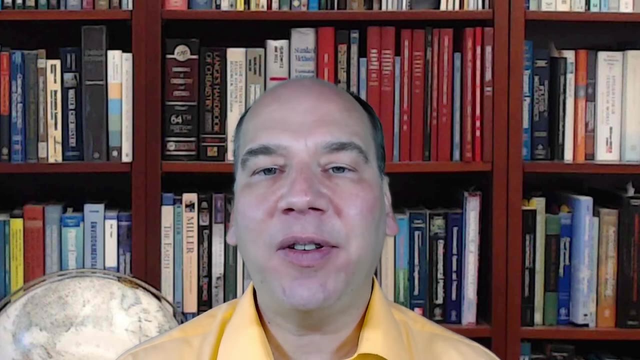 should really always keep track of s surroundings, s system and s total, but we can get sloppy about that, um, and even if i'm perfect about it, which i won't be other authors and other places you encounter, it will be sloppy. so when you see that s always ask yourself: am i talking about entropy of 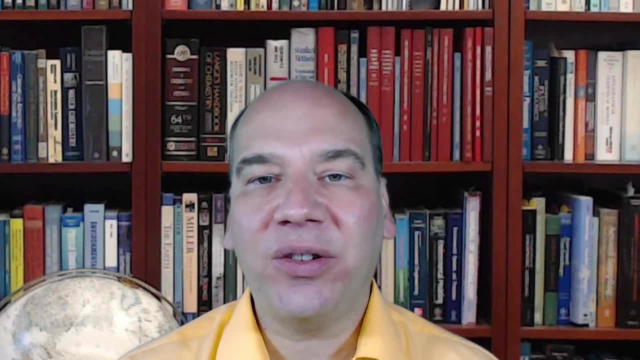 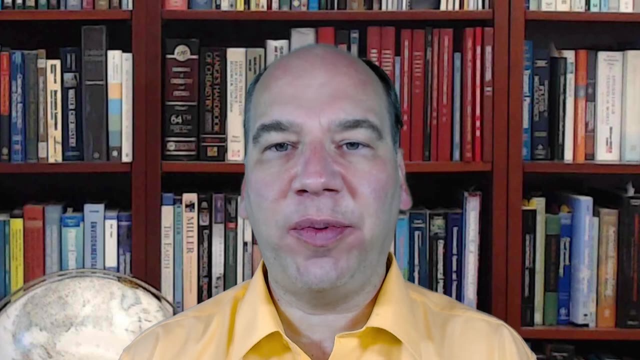 Am I talking about total entropy, S system plus S surroundings? What am I talking about? It's going to be important to always keep that in mind for the math and the messages to stay clear. Okay, let's next advance on the concept of entropy, or the use of entropy, by using a specific famous example. 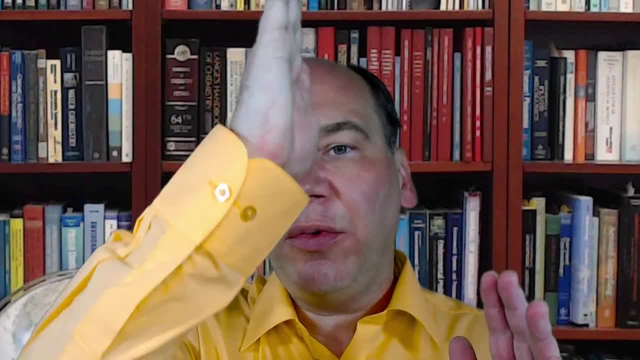 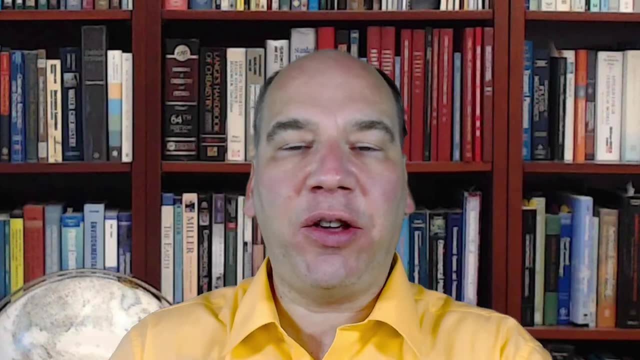 Let's have two compartments in contact. They're divided by a removable slider. One has a high-pressure gas in it and the other side has vacuum. So when we remove the high-pressure slider, we know right away that the high-pressure gas goes to the low-pressure side. 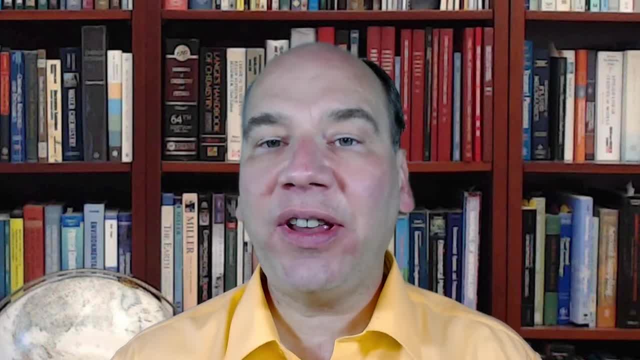 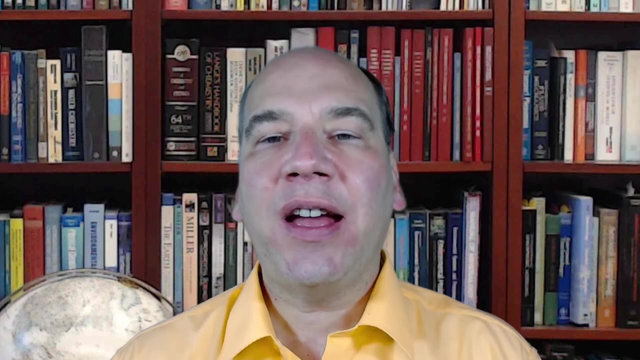 We know that's spontaneous. Let's calculate now the entropy change associated with that. We're going to say that these two boxes together are isolated from the environment. so no energy or work or mass exchange with the surroundings. So right away that means no work interaction, no heat interaction. 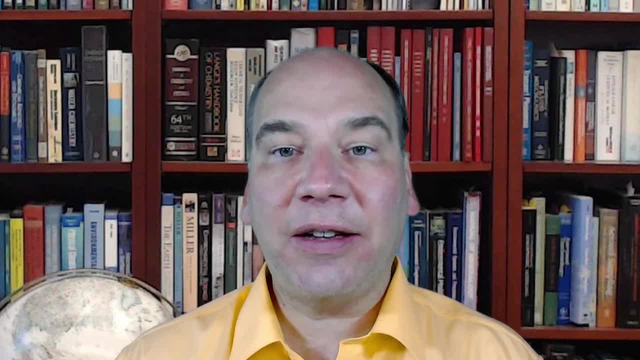 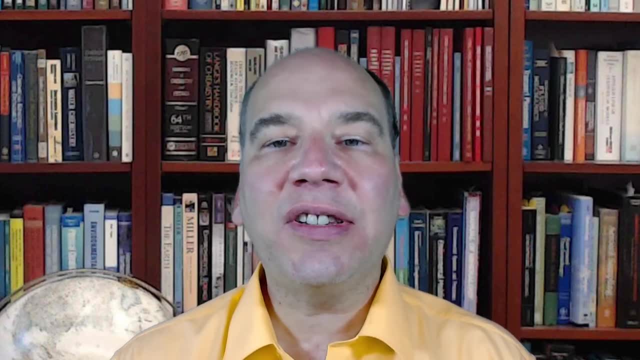 This gas expands into the other chamber, Those two chambers will be the same size and it will be an ideal gas. What we'll see is that, although that is an irreversible process, meaning that the change in the entropy of system is positive, especially because we're isolated from the surroundings- 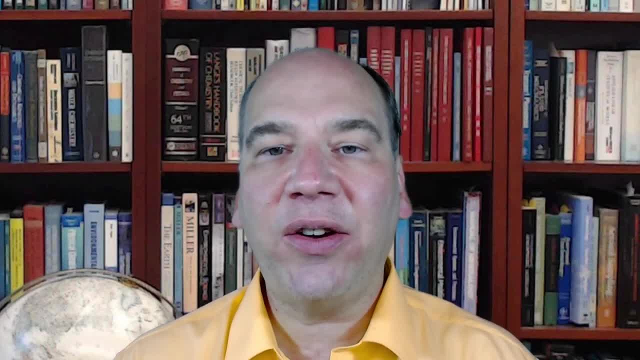 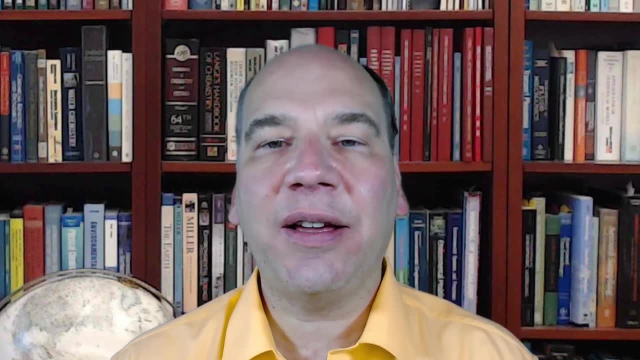 the change in entropy of the surroundings is zero. So we have those two together. The change of the entropy of the universe is positive. Our change in entropy total is positive. That's good. That's our use of the second law, meaning it's spontaneous. 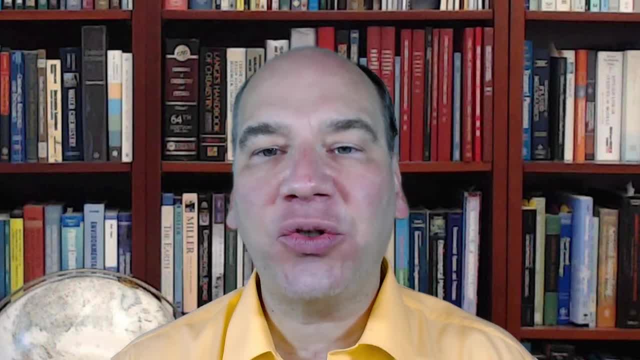 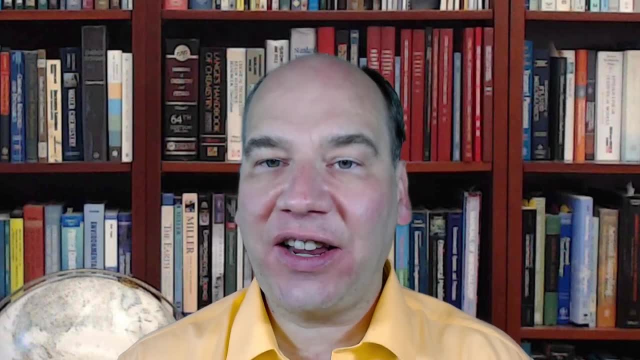 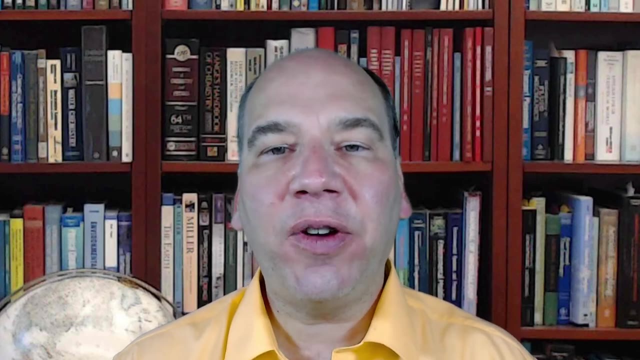 So, although that's irreversible, to calculate the actual value of the change in entropy, we will follow a reversible pathway that gets to the same destination And we'll use that reversible pathway then to calculate the change in entropy, Since entropy is a state function if we get to it following a reversible pathway. 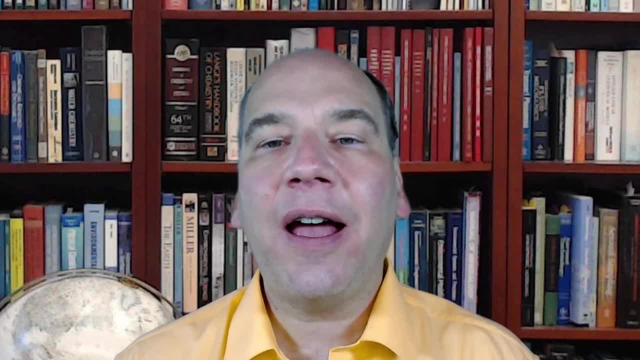 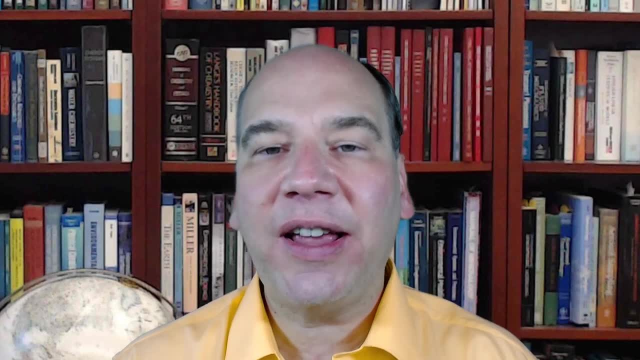 the same final state, the same pressure, volume, temperature. if we get to that same final state following a reversible pathway, then we can say that change in entropy that we can calculate on the reversible pathway is the same change in entropy that happened on the irreversible expansion. 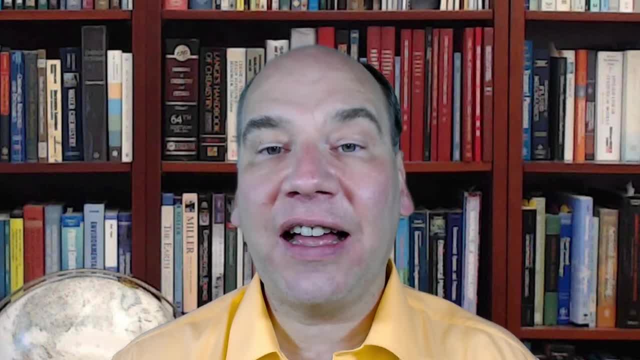 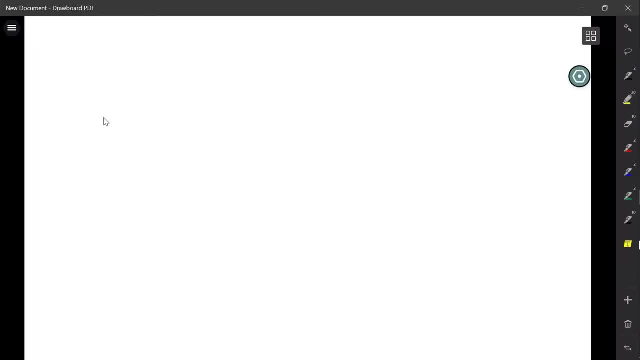 or the irreversible pathway that took place. So let's dive into that now as an example. Okay, so to dive into this, let's imagine if we have a chamber- Okay, we have a chamber, And in that chamber we're going to have 10 to the 5 pascals of what 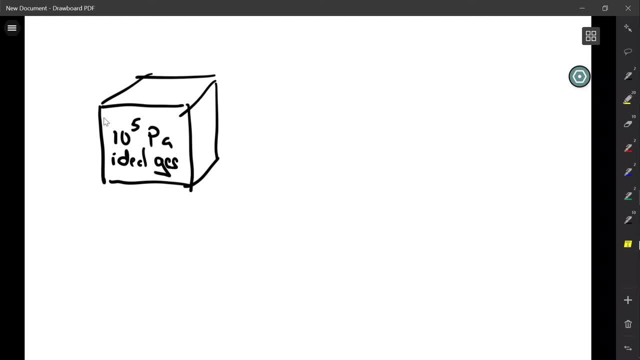 Of an ideal gas And it's going to be next to another chamber. This other chamber, in the initial state, will have no gas in it, So it'll be vacuum. We'll just put zero pascals And they are separated by a divider. 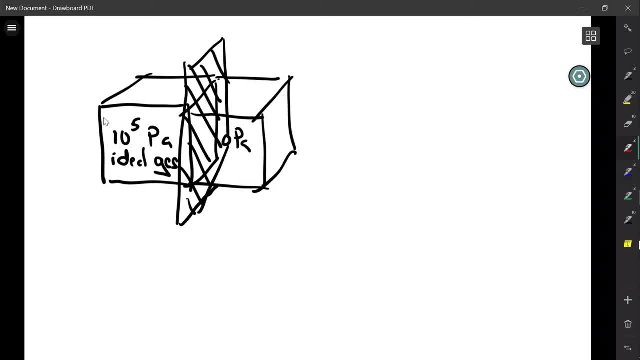 And these two chambers together are highly insulated from the surroundings so that no heat interaction can take place, And the two boxes are rigid borders, so no work interaction is taking place. So this is the initial state, And then what we do is we remove this divider. 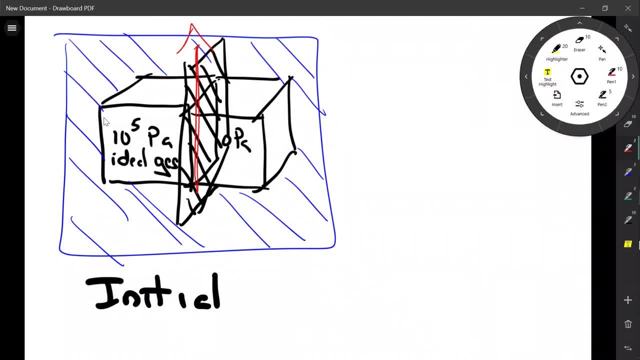 So now the two boxes are connected, And when the two boxes are connected, we have one larger box. Okay, so now we have one larger box, And if the two boxes were originally of the same volume, then the final volume is twice that. 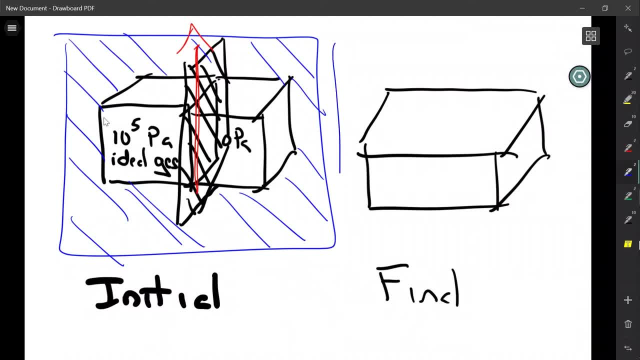 This will be our final state. This whole thing, of course, is still completely isolated. Now we can ask, given that we had kind of two systems, we had kind of system one, which was a box over here, and system two, which was a box over here. 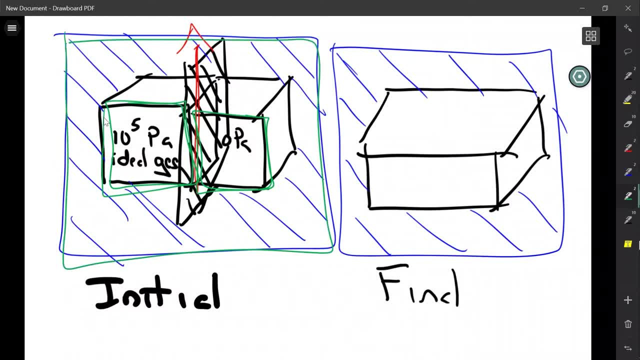 And then we have the surroundings. Well, okay, so the system and the surroundings we can see. since it was totally isolated, when we went from initial to final, there was no heat interaction. because it's totally insulated, There was no work interaction between the system and the surroundings. 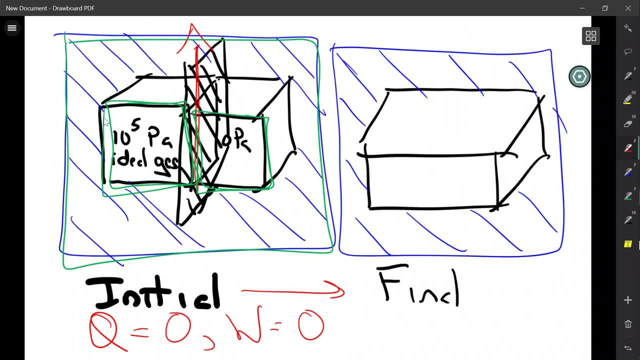 That's okay Between the two systems when we remove the two boxes. when we removed that partition, we also weren't pushing against anything. We also weren't having any heat interactions. So when we're done, then we can ask what's going on over here in the final box. 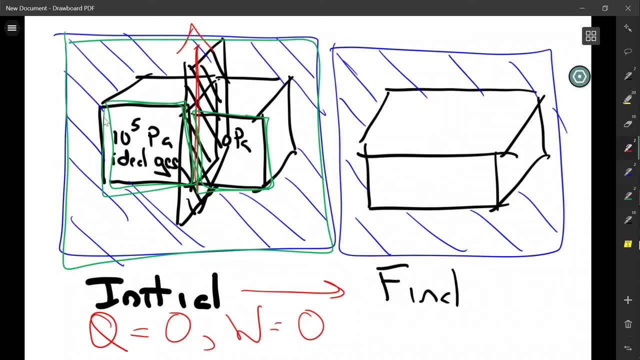 with regard to pressure, volume and temperature. Well, for an ideal gas, we have a couple of things. about the ideal gas One, we have its equation of state, which is: PV equals NRT. The other thing about an ideal gas: 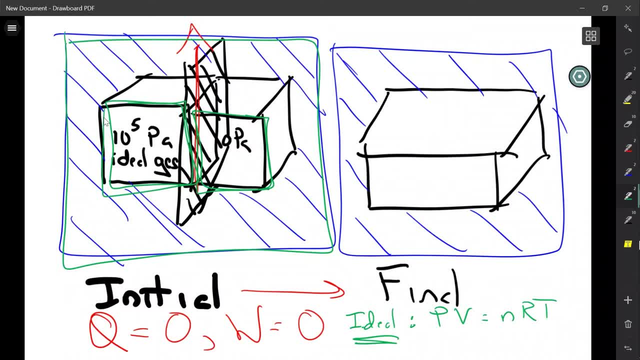 is that its molecules don't have any interactions, And so the relationship between its internal energy and its change in temperature is a constant relation, meaning that the internal energy of the gas only depends on temperature, That heat capacity has no dependence on the density of the gas. 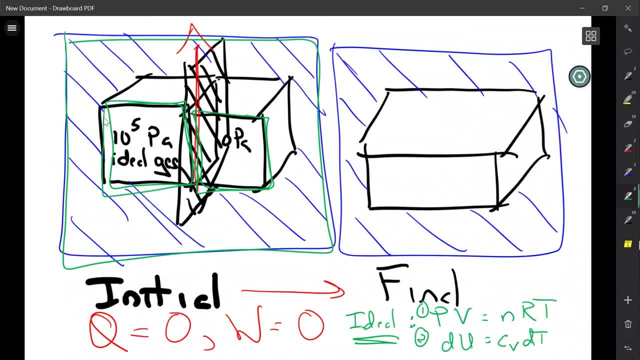 because it's an ideal gas. It's a property, part of the definition of an ideal gas. So if we look at that, we can then say, well, okay, what was the change in energy? Well, the change in energy should be Q plus W. 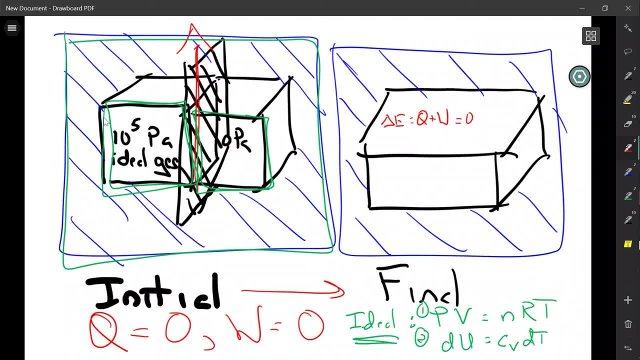 which is zero. And the change in energy? when we have no kinetic energy, gravitational potential energy, the only thing we have is possible internal energy. So the change in internal energy must also be zero. And since the change in internal energy is zero, 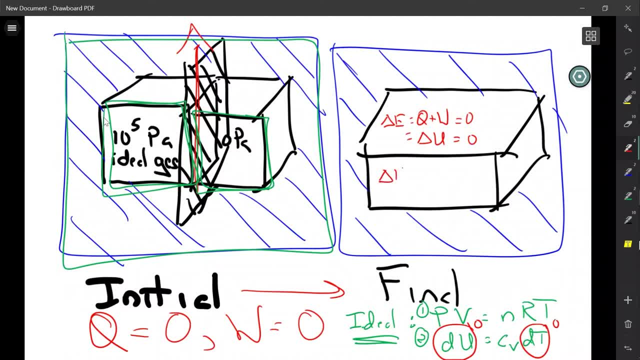 then the change in temperature is zero for this ideal gas. And since the change in temperature is zero, then this term in the equation of state is a constant. So pressure times volume is a constant. So that means that if the volume went up, 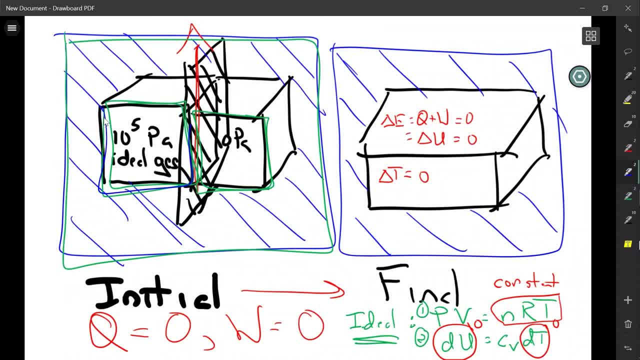 because I said I had two initial boxes of the same volume. if the volume doubles then the new pressure- since PV equals a constant- the new pressure must be half of the initial pressure. So that is the expansion of an ideal gas into vacuum. 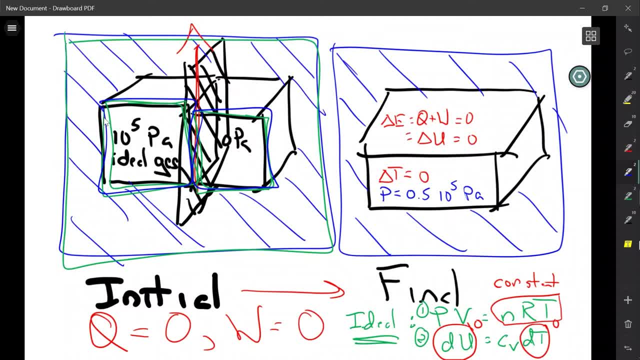 no change in temperature and the pressure goes in half. Well, again, we know that must be irreversible. It must be irreversible because that gas will never spontaneously separate back into a region that's at high pressure and low pressure. So we know from common experience. 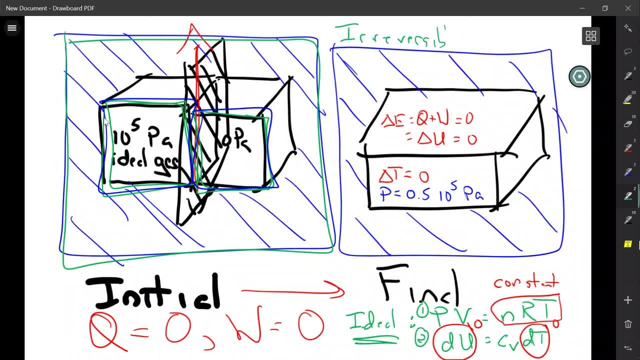 this must be irreversible process. irreversible process or irreversible pathway was followed. So then the question emerges, the one, the question we really want to answer, then, for all of this is delta S, the change in entropy is what Delta U was zero. 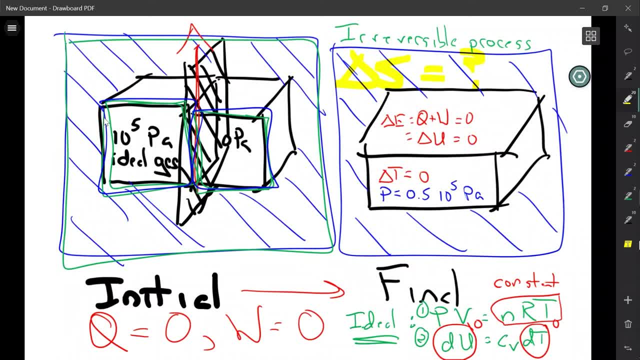 delta T was zero, but the process was irreversible And, to be specific, in this case, delta S. well, we're delta S. just to be specific, is delta S of the system right? Delta S of the system, We know delta S of surroundings must be zero, since it was an isolated. 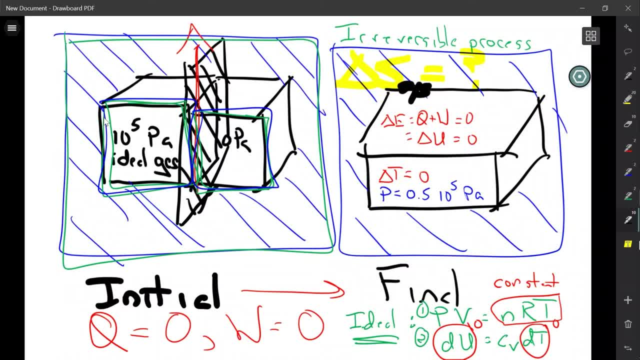 no interaction. So we look for delta S of system. in this case we're also asking what's delta S total? So how do we answer that? Well, we're going to go to the next slide to answer that, to get the delta S quantity. 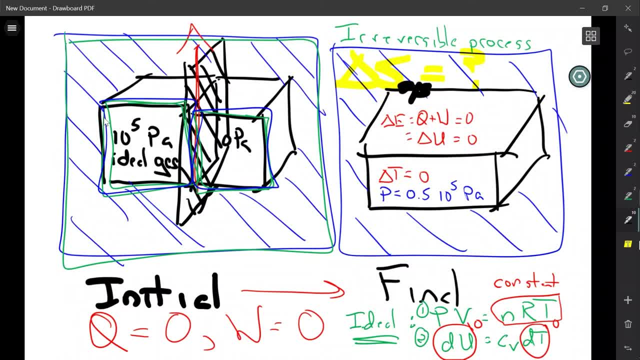 We have to do the same process, meaning we should end up with delta T of zero, a pressure of one half. We're going to get to that same destination starting at the initial state, going to the final state. We want to get to that same destination of delta T equals zero and pressure. 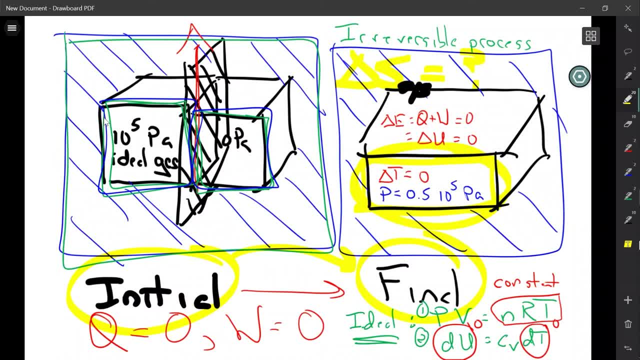 equals half of 10 to the five PA for doubling in volume. We're going to get to that same destination following a reversible pathway And then we'll be able to calculate delta S of system. by using along that reversible pathway we'll be able. 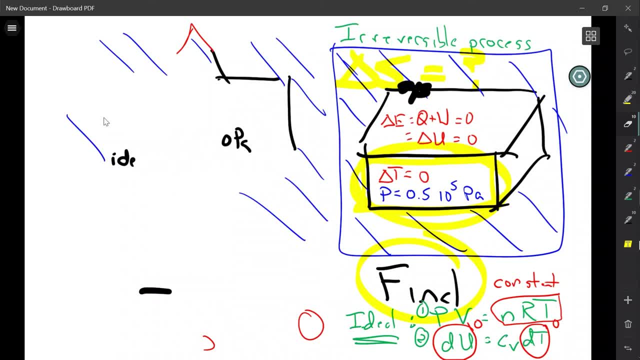 we'll be able to use along that reversible pathway. We'll be able to use our definition of DS, of the system equals heat interactions, reversible over T. We'll be able to do that and calculate the S and because S is a state function, 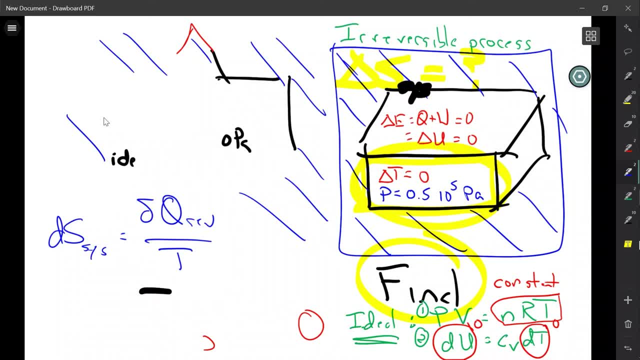 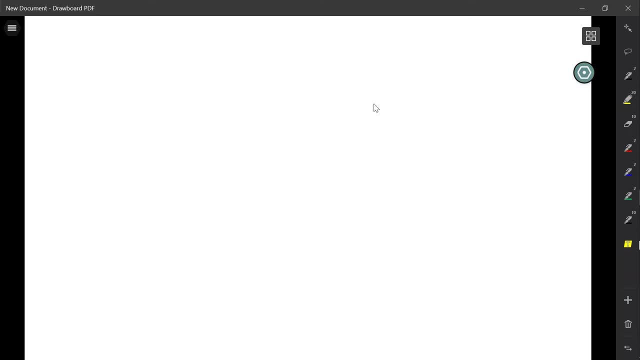 we will then know what the delta S was By getting that same destination by an irreversible process. So let's go ahead and do that, Okay, so our goal here is to go from this initial pressure, which we'll call P initial, which was 10, to the five Pascals and this initial volume. 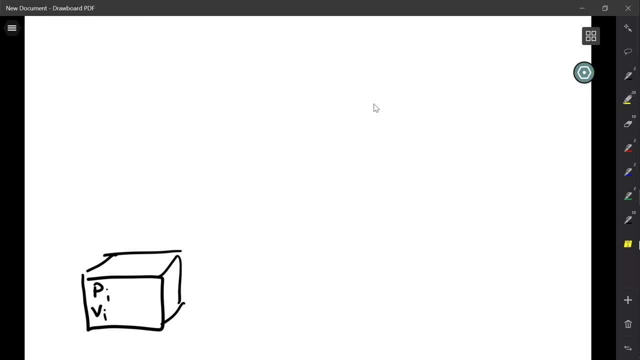 which we'll call one cubic meter, and this initial temperature, which we'll call 298 Kelvin. So 10 to the five Pascals, one cubic meter and 298 Kelvin, That's going to be our initial state, And we did this irreversibly. 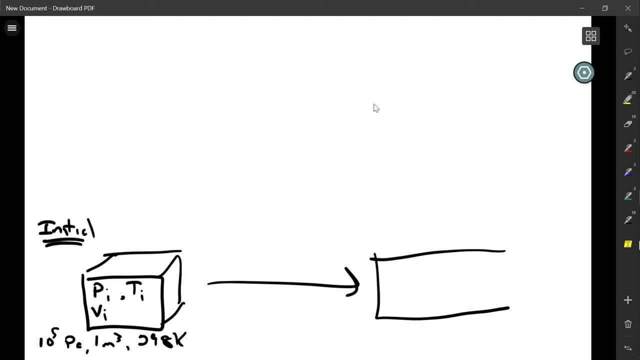 We got to something that was twice the volume. So P final, V final and T final. We know that it's twice the volume and the P final was one half the initial value, 10 to the five Pascals. The V final was twice two cubic meters. 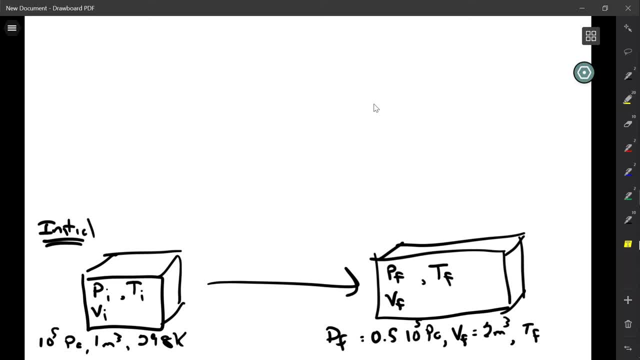 The two, one to two is doubling the volume and the temperature didn't change. Now we did that irreversibly and we're trying to find out now what is the delta S of the system for that process to get into our final state So graphically. 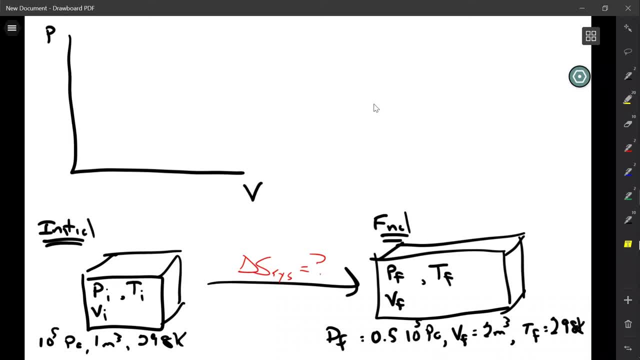 we start with a pressure volume and our working fluid, so to speak, the gas, the working fluid, which is a technical term. the working fluid, the material, was the ideal gas, And that's the equation of state for the working fluid of the ideal gas. 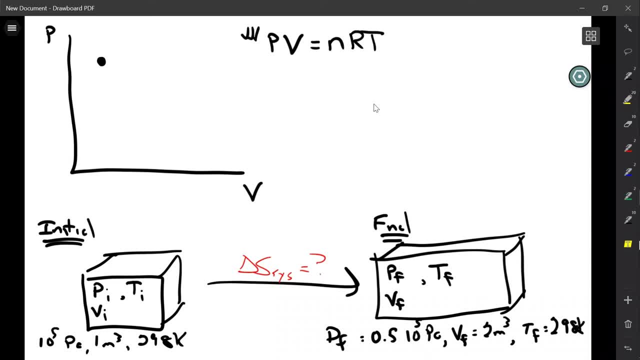 So if we start at some pressure and volume and we're moving to a final pressure and volume where the volume doubled, well, based on the equation of state, PV equals NRT. if we stay at constant T, that would be, PV equals a constant. 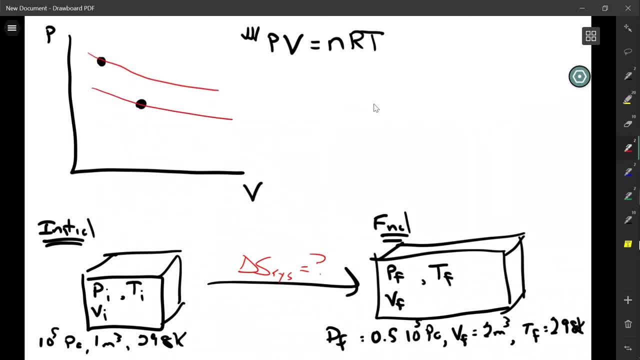 So we can draw isotherms. Isotherms meaning constant temperature lines, That's where PV equals a constant, or meaning that T is a constant, meaning that delta T along those lines are a constant. Okay, So if we consider then, 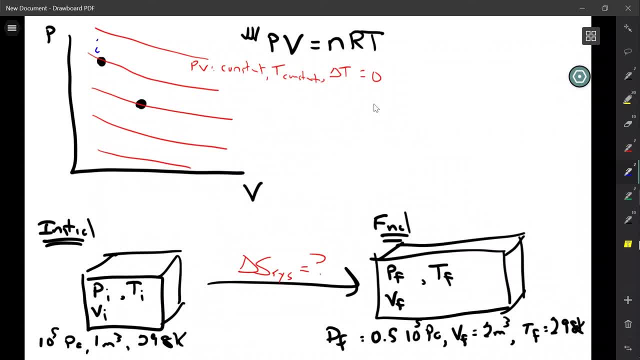 the initial state here. we should stay on that line as we try to move to our final state. So if we're doubling the volume, we should be moving approximately this way. Okay, Approximately that way. That was our initial and final state. 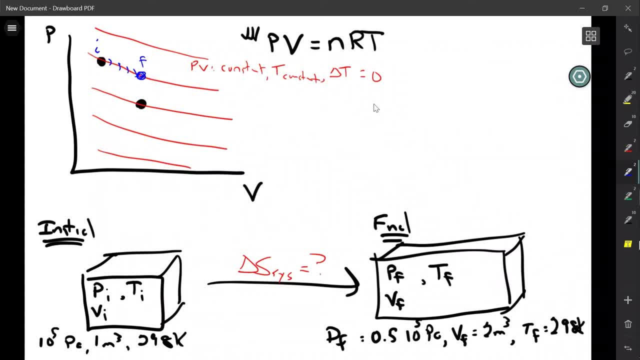 So how can we think about doing that in a reversible fashion? Well, we could choose first to allow no heat interaction, Just to get ourselves to the right volume. So no heat interaction is what we'd call an adiabatic change. So you go down here kind of in step one. 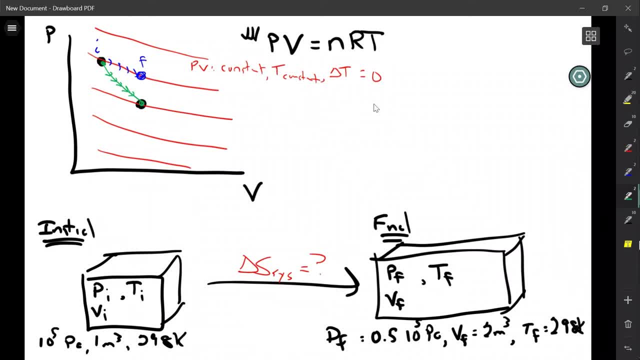 if we could do that, reversibly expanding the gas but not allowing any heat interaction with the surroundings. If we do that in step one, then in step two we could stay at the same volume and have a heat interaction apply fire. 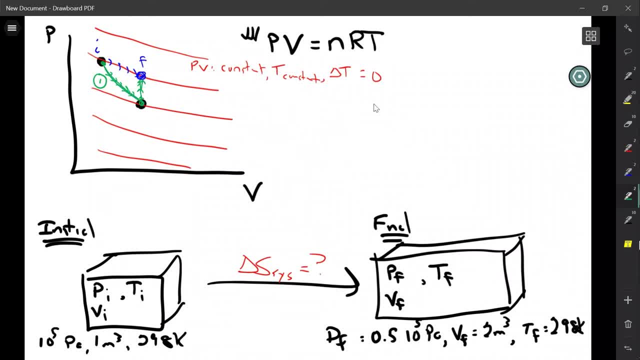 Okay, So we're going to. we're going to do this in step one, step two. we're going to do that on the next slide, And I drew those as solid lines just to indicate that we're actually following a reversible process. 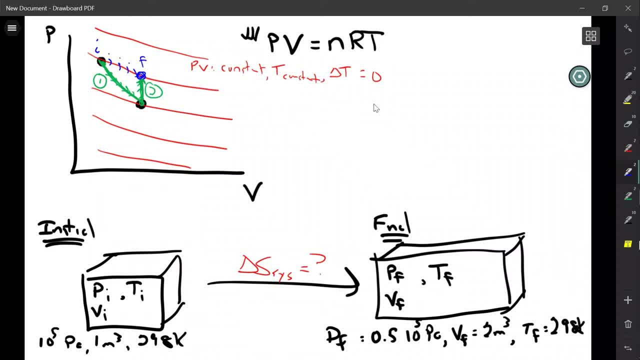 Whereas these kind of pointy blue lines just means we change. but we didn't really have pressure and volume controlled. We didn't really know what they were. It was just a rapid expansion, So certain pockets of the gas were probably higher pressure. 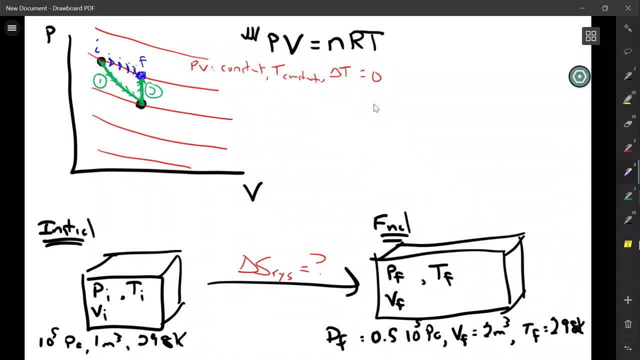 Some were probably lower pressure. We can't define a pressure statistic, So somehow we just jumped from initial initial to final for the irreversible process, Whereas for the reversible process we were able to follow these smoothly changing lines, And we're going to do it in two steps. 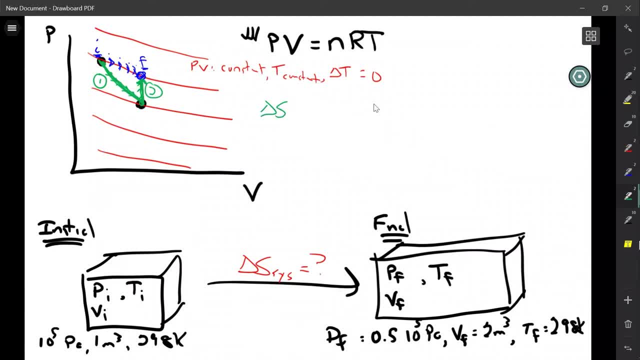 And we're going to calculate for them The overall change. Delta S, a system, initial to final, is going to be the Delta S of the system for the first step, which we'll do irreversibly, plus Delta S the system for the second step. 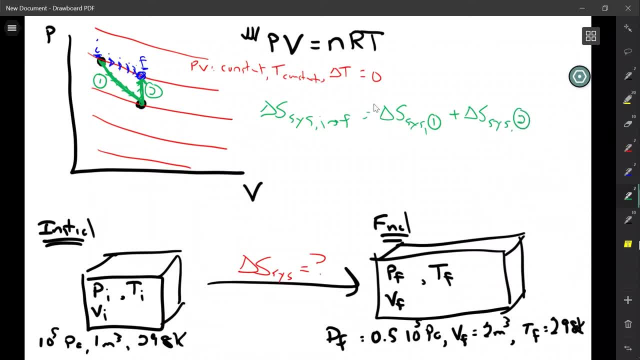 which we'll do irreversibly, And then whatever we calculate- calculate there for the reversible steps- must then also be the same value as for the irreversible pathway, for which we couldn't do the direct calculation. but S is a state variable, So we're okay to do it by a different pathway, as long as we get to the same final state of pressure, temperature, volume for the combined reversible pathway compared to the irreversible pathway. 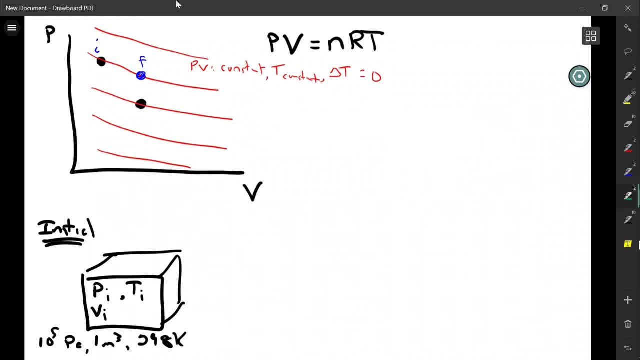 So let's dive into that. So in the first step, we want to move on a well-defined path one, and that well-defined path one which proceeds as follows: So it's going to be doubling the volume under the constraint of an adiabat. 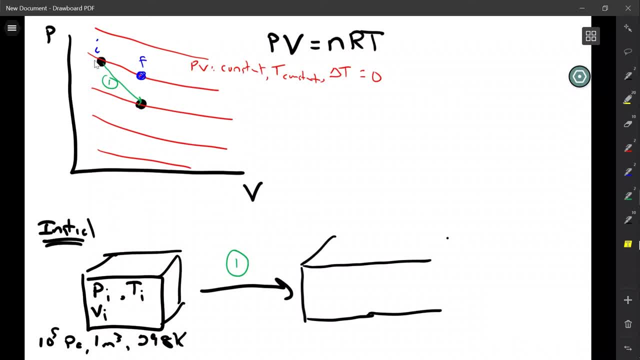 So if we are doubling the volume under the constraint of an adiabat in step one, where an adiabat, when we say that word, that means that the heat interaction, in this case the reversible heat interaction, is zero. Okay, so I'm going to move pressure and volume while having no heat interaction. 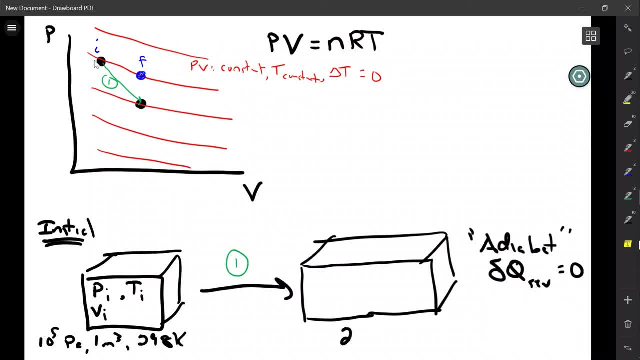 Well, when we're all done, then by definition, I want to double the volume. I don't quite yet know the pressure I I could calculate it, but I haven't yet done that for you. I don't quite yet know the temperature. 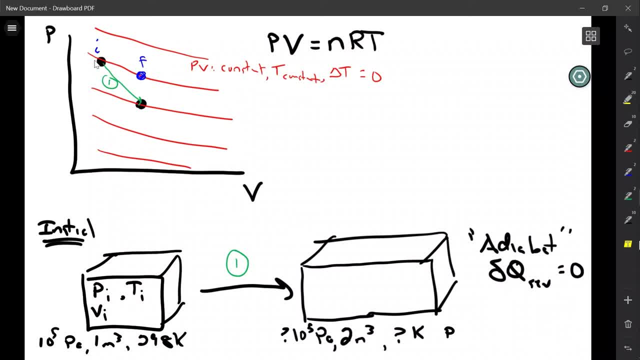 I could calculate that but I haven't done it for you. But we do know that PV and RT, when we doubled the volume, that equation of state must still be followed, even though I haven't quite given you the pressure and temperature. But more importantly, 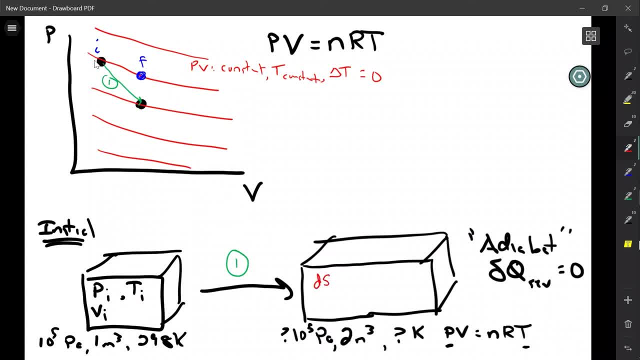 given the definition of DS of the system and given that it's the adiabat, we can't say that it's zero. Well, we've just said on the adiabat that this is zero. So if we then integrate across, across the whole business to get the change in the entropy of the system in step one. 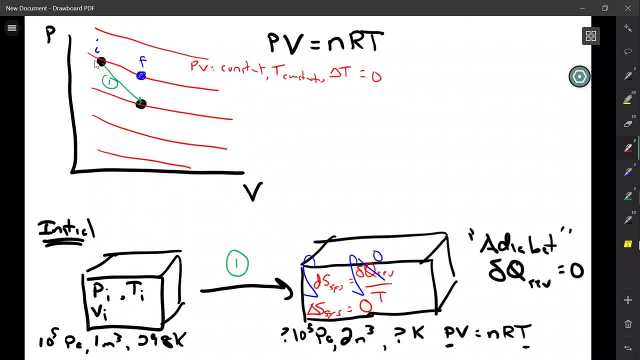 well, that's just got to be zero. So we have figured out that for going along the adiabat from along this green line, that for this part, number one, tell the S of one for the system is zero, because we're following the definition of the adiabat of no heat interactions. 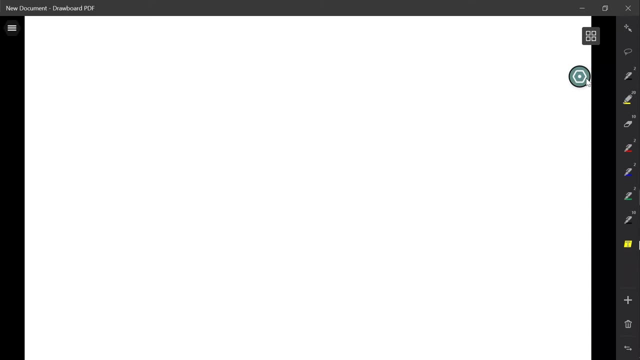 So, as we move along that adiabat and we want to know what those final temperatures and pressures are, well, we're gonna have that: the delta change energy of the system. in this case, the only term there is, it's it's internal energy. 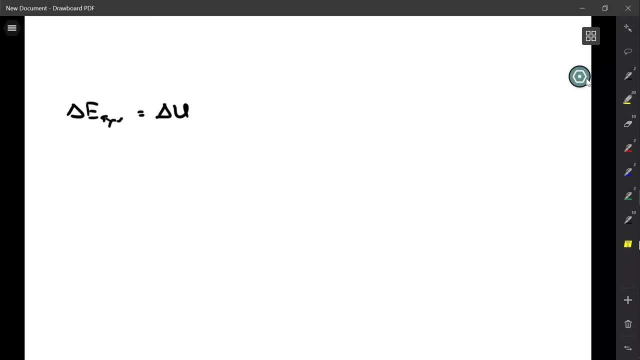 no kinetic energy and so on and so forth. If we do that on a differential basis, then we should have that. they change internal energy as a CV times DT, Since it's a ideal gas if you want to do it on a molar basis. 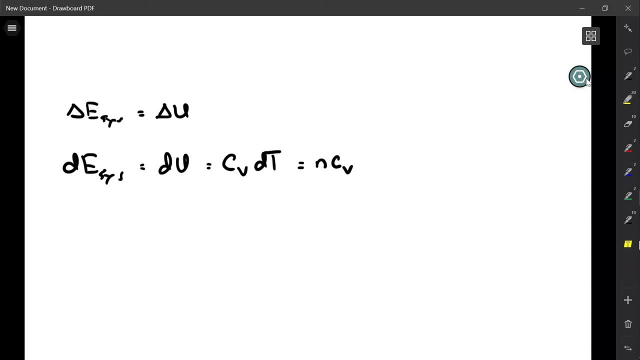 we can put in the number of moles and these a little CV instead of a big CV where that's the heat capacity per mole, And that energy change should be balanced by whatever heat interaction and work interaction we have. Well, we said by definition, 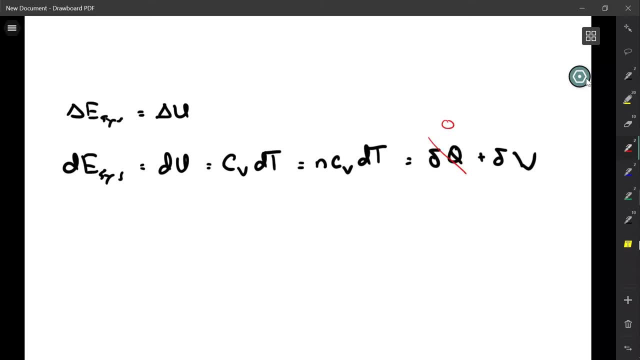 we're on this adiabat, So the only thing we have left is a work interaction, And if that is we're expanding, we're doing pressure against a volume, So the work term is just negative. P DV, That's the force acting through the distance. 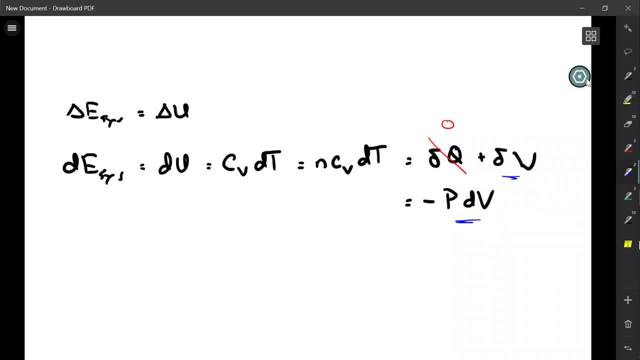 And the system loses energy and negative as it as it pushes against a pressure. So we also have the ideal gas law which we can substitute in for a pressure. PV equals NRT, So that gives us negative P. I'm sorry, It gives us a PV equals NRT. that gives us a P. negative NRT divide through by V DV. 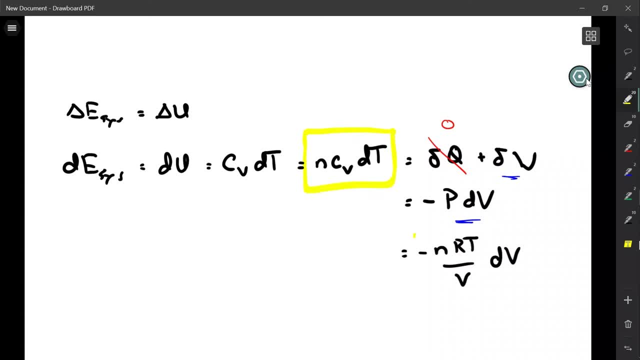 So we've we've managed to equate this with that, And so if we rearrange that, all the ends cancel so we get N CV D, T equals negative. N RT V over DV- the ends cancel. We rearrange the terms so we can write D T over T: equals. 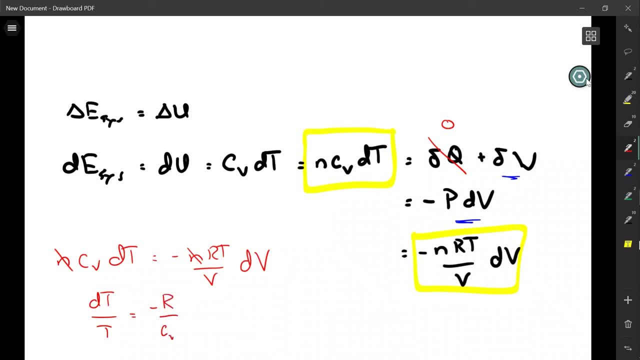 uh negative R gas constant over cv, dv over v, and then we can then integrate that from our initial temperature, which we knew, 298 kelvin, our final temperature, which is what we're trying to find out, our initial volume, which we know is one cubic meter and we doubled it. our final volume two. 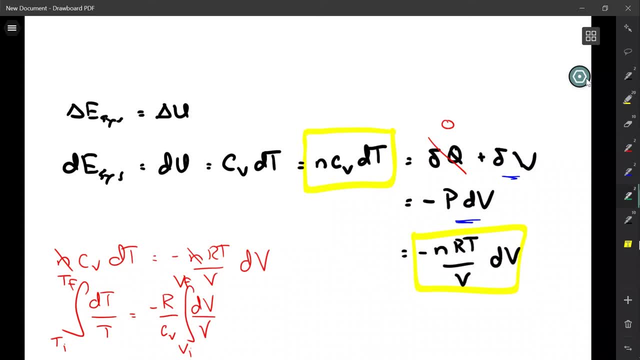 cubic meters. that was part of the description and so if we integrate those, we end up with the relationship where we can now find the final temperature: tf d final over t initial is v final over v initial raised to the negative r, c, v. okay, now we could do that out, but the 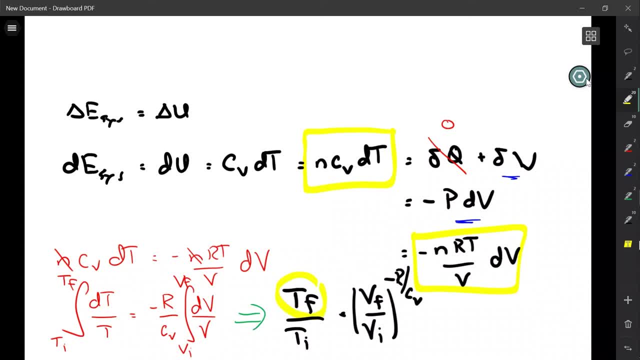 important point here now is we've got tf in terms of things we know about, the initial temperature and the final temperature. so we can now find the final temperature and the final, the initial volume and the final volume, and then cv for our ideal gas and negative r. so tf now is a defined quantity. when you get to the end of that adiabat, doubling the 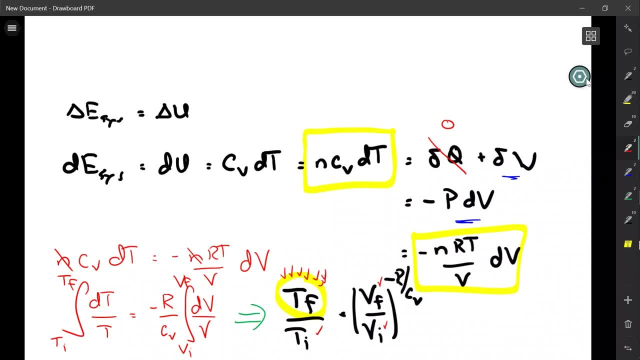 volume. put another way, we now know delta t as well. if we wanted to delta t what the temperature change was? again, i'm not calculating this with real numbers. you could just substitute in the initial one cubic meter v, final two cubic meters t, initial 298 a, kelvin, gas constant and the heat capacity. but we can. 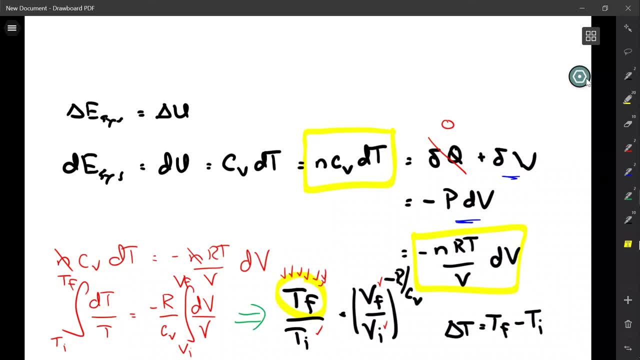 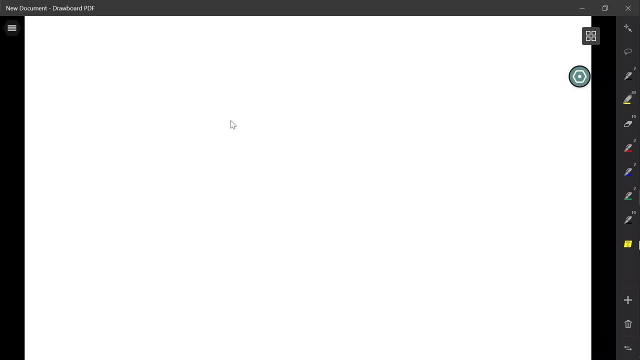 also get the delta t from the start to the finish along the adiabat. that's constrained to that doubling of the volume. okay, just as a specific example, following up on that equation, from the t final, well, it would be t initial, v final over v initial. 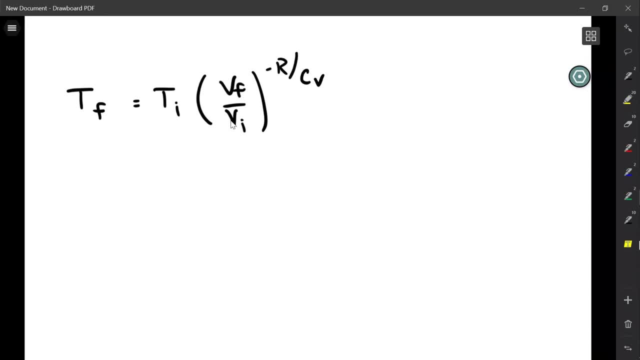 zero and then cv c plus negative r, combined again right. so now we can just multiply that with the heat of quake. now, this here is a very important thing- just putting the combined elements here- but also a very important feature of this solution that we can above root over this step of g. so we can get this using this checkerboard. 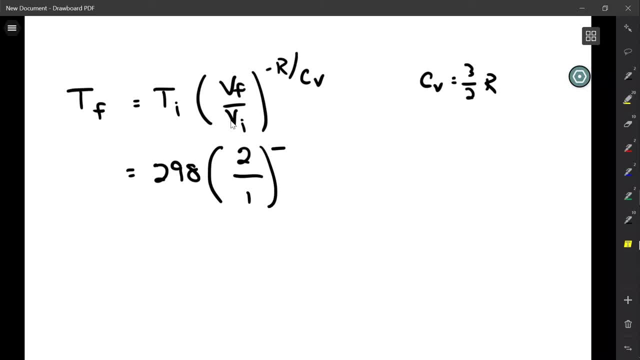 function: unit expression: 150: 0. all right, so let's go ahead and take a look at this1286 questionER喂. and here we can see that if houste with the end and end units of e zero is equal ك divided by three-halves R, well that's negative two-thirds R and then. so if we- I'm sorry, 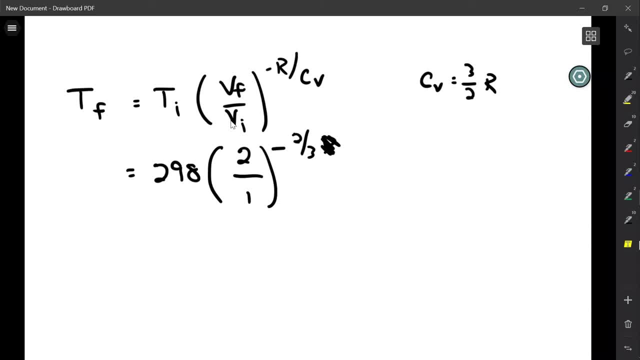 the R cancels out, that's negative two-thirds. so if we then evaluate that for its final value, then we get 187 Kelvin. So in that expansion, our adiabatic expansion, from our initial point to our final point, with no heat interactions but pushing and doing work on the outside and 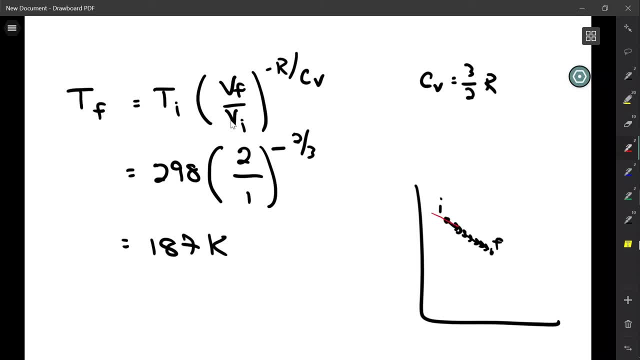 therefore losing joules. we crossed from an isotherm of 298 Kelvin over to an isotherm of 187 Kelvin, And so our next step is going to be to push ourselves back up to our final point that we got by the uncontrolled expansion while holding volume. 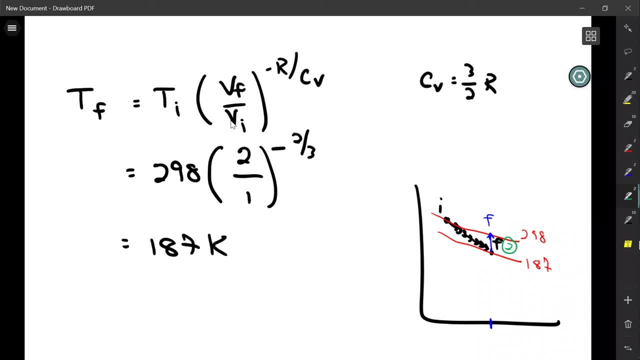 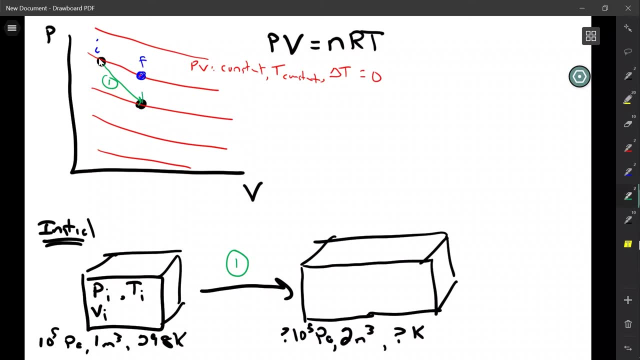 constant. So that'll be our next step. step two, Now the next step. we have gone from along one, so now the next step. we want to get from here to here in step two, in step two. so the idea is that in step two we can get to our target, which was the final state we got to. 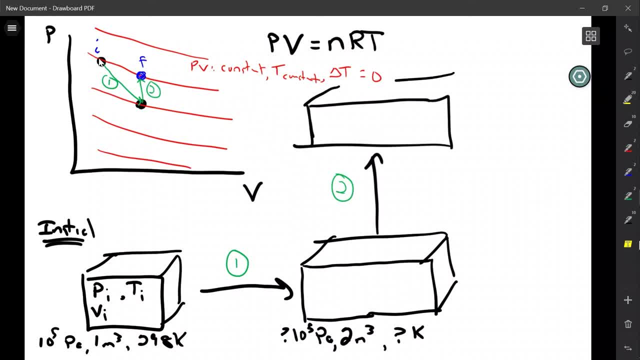 in the case of the irreversible, which was that we have now the known volume again. the volume has doubled to two The pressure. well, we know what that is. now it's one-half, and then the temperature should get back to its starting point, 298 Kelvin. 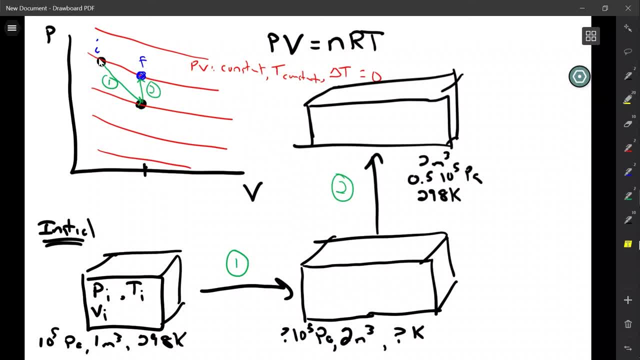 So this transition two is being done at constant volume. dV equals zero. we call that an isochore. So we want to know the change in entropy of the isochore and we can see that we're staying at the same volume but we're increasing temperature. 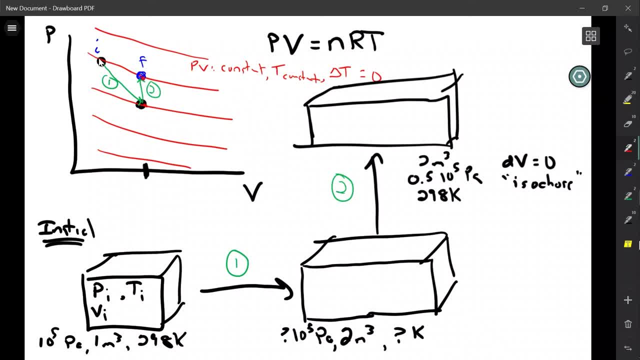 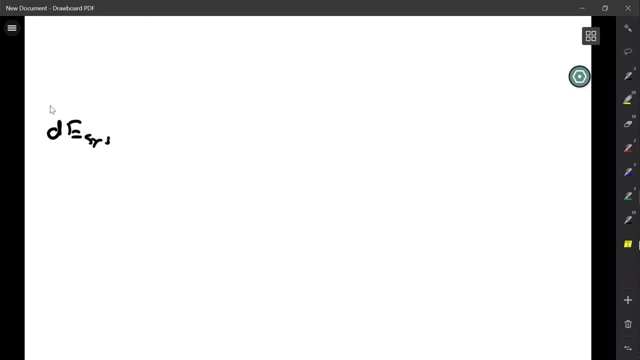 So the governing equation for this would be as follows: The incremental change in the system energy again is just the internal energy, because there's no kinetic energy, gravitational potential energy and so on, And we know that for the ideal gas on a molar basis we've got n little c dV. 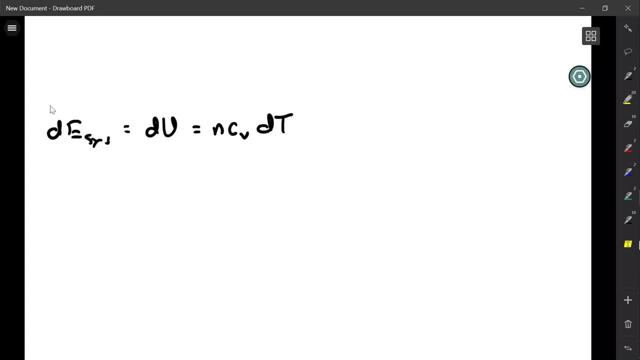 heat capacity, dt, and we further know that that should be balanced against whatever small amount of heat interaction there is and whatever small amount of work interaction there is. now, because we're on the isochore, the PV work. well, there's no change in volume. DV equals zero. so there's no work, so it's. 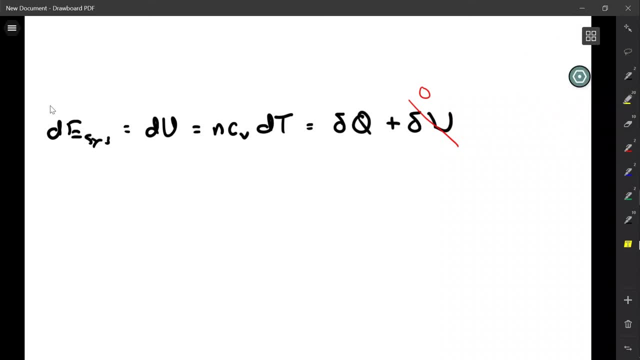 all tied up in the heat interaction. okay, well, as we're doing all this reversibly, we know that the change in entropy of the system is the heat interaction reversible over T. we're doing all this reversibly so we can replace the heat interaction here with T DS system. and now we can take this part. 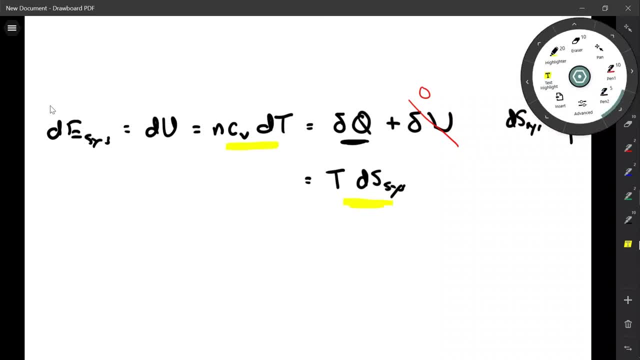 of the equation, this part of the equation and this part of the equation, and we can connect them. so we get that n CV DT equals T DS system. we rearrange, we get that DS system equals n CV DT over T, which we can then integrate. that leads: 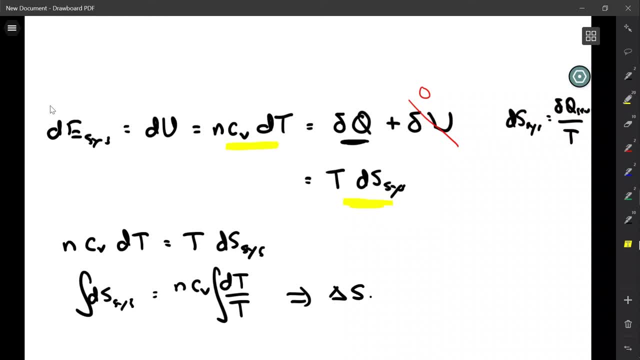 to the change in entropy of the system is N? CV, from the initial temperature, which in this case is the initial temperature on segment two, to the final temperature on segment two, DT over T, which leads us to the natural log relationship nCV. then there's natural log t final over our t initial, where that's on segment uh two. okay, we're now getting. 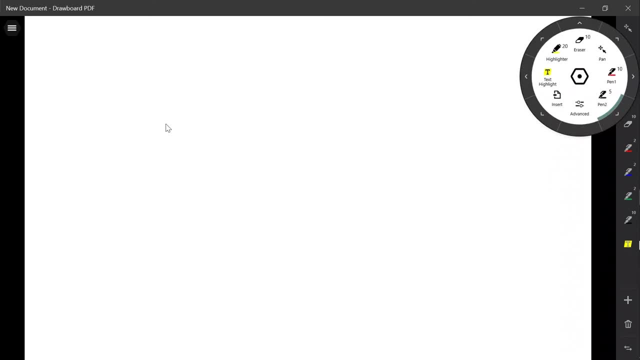 very close uh to being done. we we obtained that. the change of the system and going from one uh to two was just uh n c v natural log of t final of segment two over t initial of segment two. now we can just do some notation things here where t final segment two by our problem. 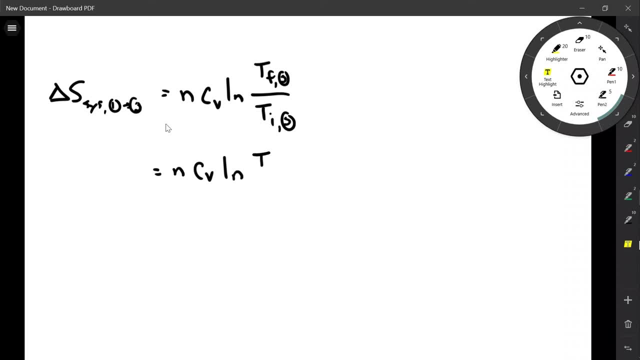 definition. the temperature didn't change from the initial, so we have that's based on t initial of segment one is equal to t final of segment two. that was part of our problem setup. that was a, so to speak, a given, and then t initial of segment two. well, that's t final. 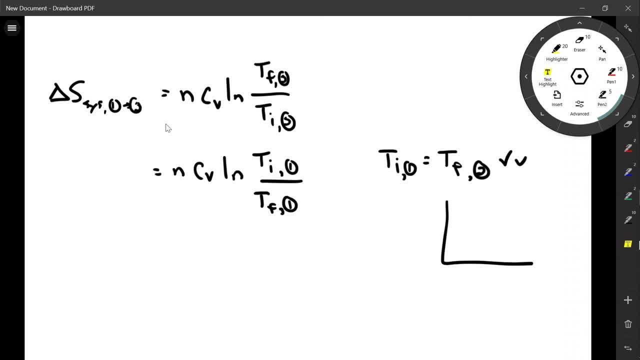 of segment one. that's based on the fact that we went from segment one and then to segment two. so what is the final? for segment one is the initial for uh segment uh two. now we also obtained the relationship of t i and t f for that segment. 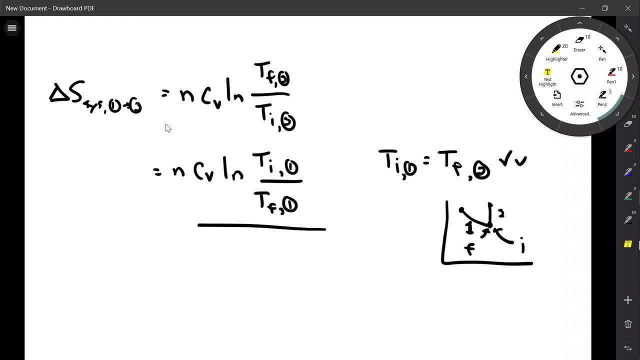 one. that relationship that we obtained was that t f over t i for segment one was the volume final over the volume initial, to the negative r c, v. we obtained that a few minutes ago, so taking that result and substituting it in, uh up here we get that delta s system. 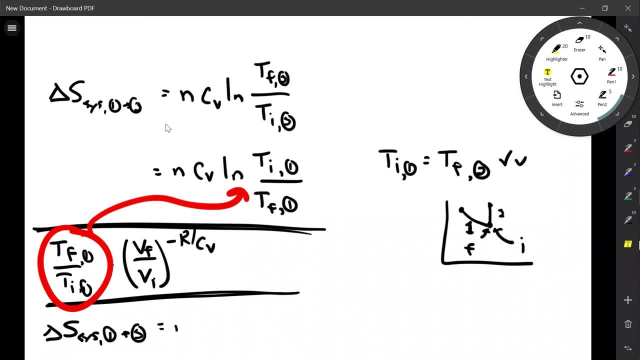 from one to two is n? c, v? um, v, f over v? i. and because we have to flip the uh, f and i, we have to substitute the i and f? um. the law of uh, uh, logarithms, uh, let's see here, i just left out a natural log in here. the law of logarithms is that we swap this negative sign. 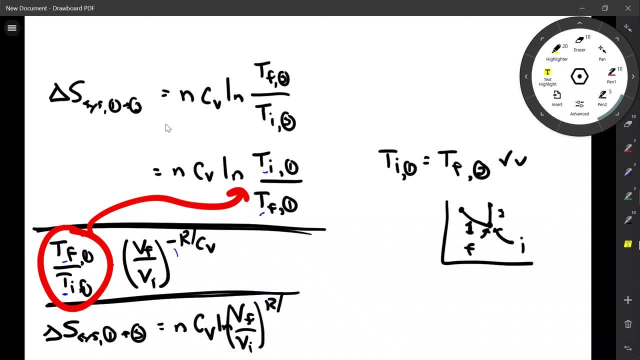 with a positive sign. so we get r c v. and then the next law of logarithms is that we can take an exponent out front in front of the logarithm. so that leaves us with uh n c v, r c v, the cv's, cancel natural log v final over v initial. and so our 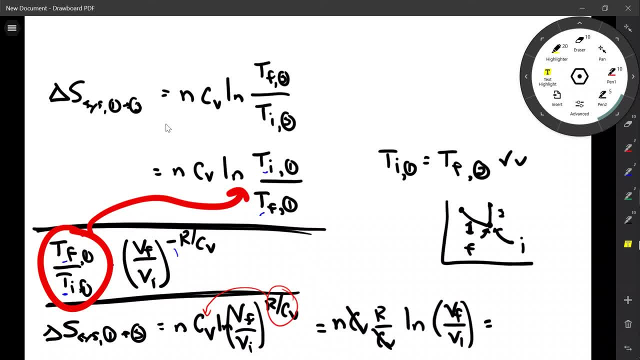 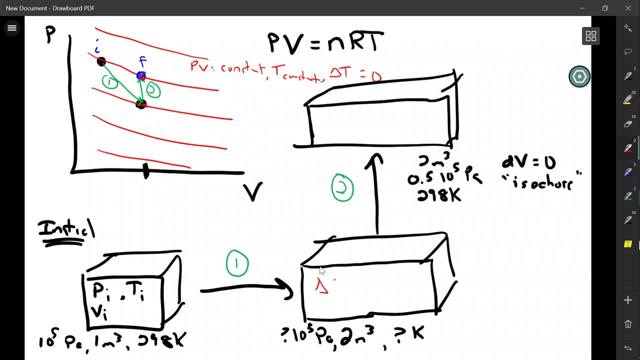 final answer for segment uh two, delta s is n? r natural log v final over v initial. okay, so now we're all set to uh calculate the total change where the change in entropy of the system in step one was just uh zero and the units on that. 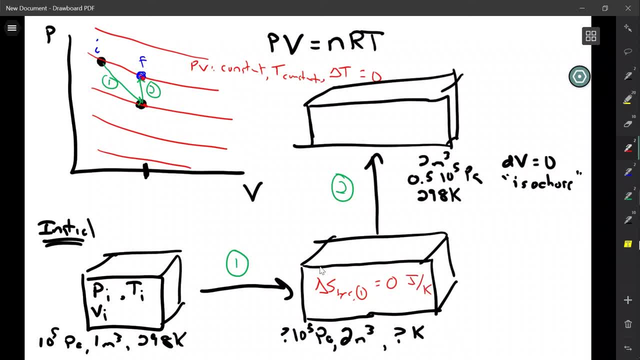 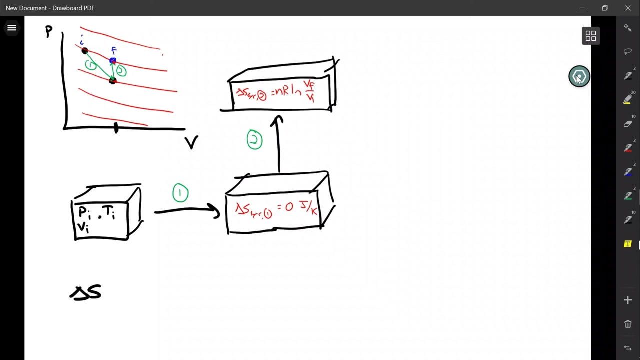 for entropy are joules per kelvin. that's where we count it. we calculated the change in entropy of the system for uh step, uh two, which we got was n? r natural log v final over v initial, so to get our total change in uh entropy. well, that total change in entropy is delta s total uh of the system. 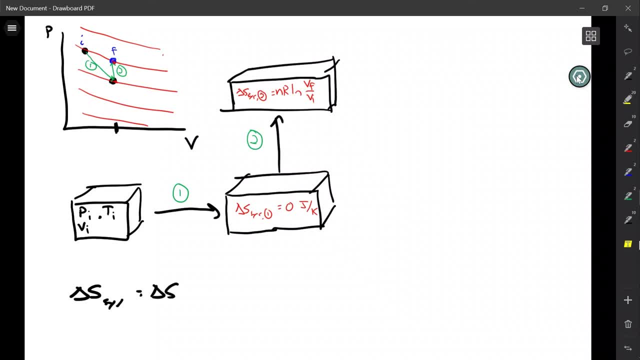 delta's total. the system was its delta s system one plus delta s system two. delta s system one is just zero. delta s system two is n r natural log, v, f over v, initial. so putting in real numbers, you're in real numbers, zero nr. well, we have, pv over t equals nr from the equation state for the ideal. 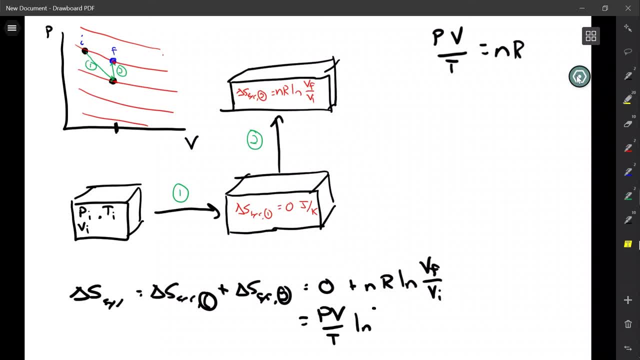 gas. so pv over t, natural log v, final over v, initial. well, pv over t. that's an equation of state. we can choose it: the initial state, final state. taking the values of the initial state, it's 10 to the 5 pascals, one cubic meter. you multiply a pascal in a cubic meter, you get a. 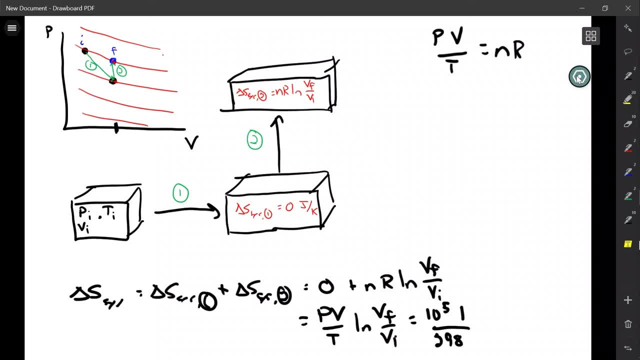 temperature was 298 and we said we were doubling the volume and if you do that out numerically you get 232.6 joules per kelvin as the change in the system entropy. so the system entropy increased- as an aside, since we did this whole thing- reversibly. that means that the total entropy system and 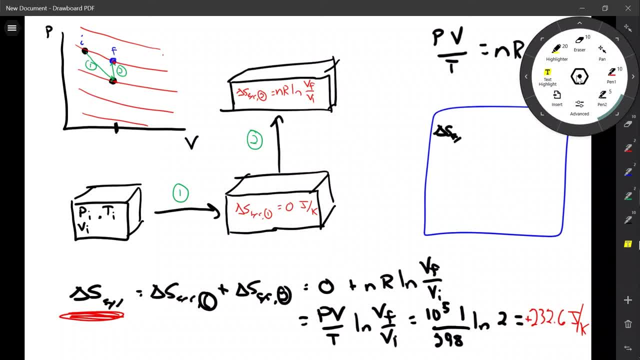 surroundings system and surroundings. so total entropy of the universe system and surroundings system and surroundings. well, that total change, since it was done reversibly, must be zero, implying that if the system is positive, 232.6, to than the surroundings negative 232.6. so in this, 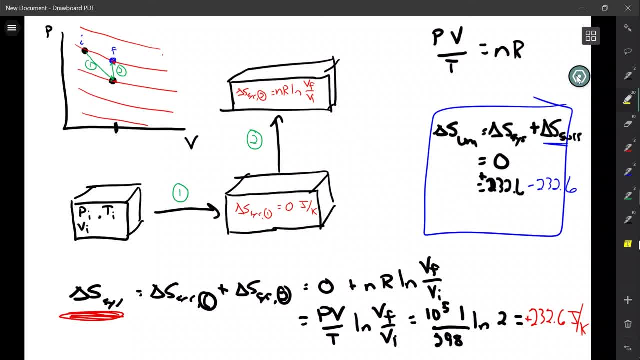 expansion done reversibly. will we increase the entropy of the system by 232.06? we decrease the sulla surroundings by negative 2.6 reversibly, the irreversible one. we didn't actually interact with the surroundings, we just did irreversibly. we just jumped from an initial to a final. well, the system entropy is the same. 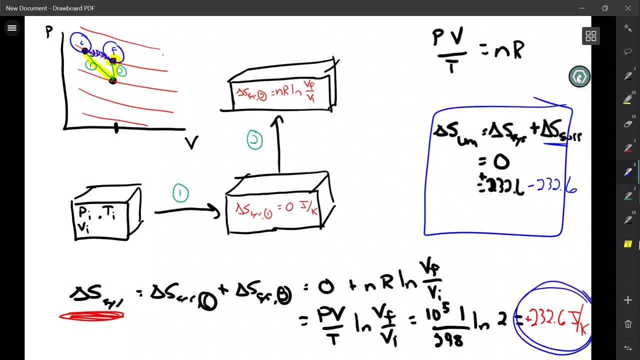 positive 232.6. the entropy and the surroundings did not change at all in that case. so in that case this was for the reversible case. in the case of the irreversible case, the entropy total change is just going to be the entropy of the system 232 and there's no offsetting change in the 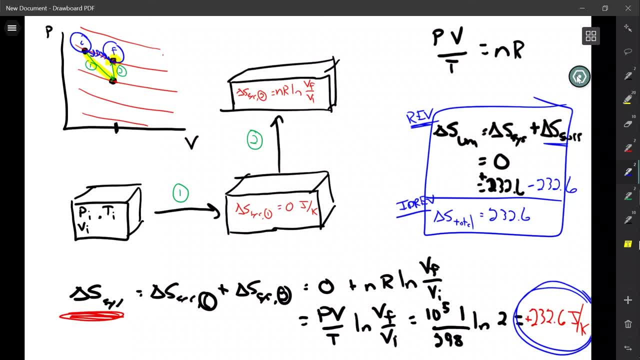 surroundings. so that's a key difference. the reversible case, the entropy the universe did not change. the increase of the system entropy was exactly offset by the decrease of the surroundings entropy. in the irreversible case, just the system entropy increased. so we see this quantity s is interesting compared to some of our other quantities and that 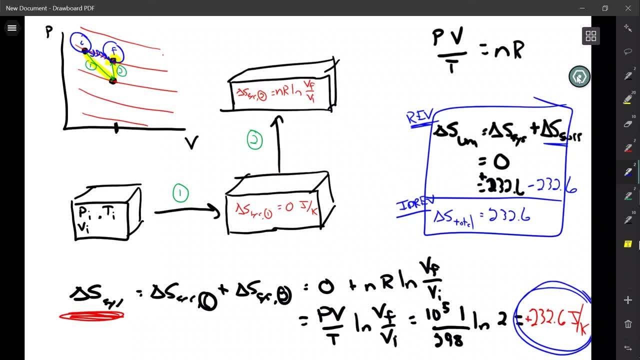 it's not a conserved quantity. you you can make more of it. the, the sum of the in the universe can't go down. you can make more of it. in a reversible case it is conserved. delta s of the universe is zero, but we have irreversible processes. delta s the universe goes up and. 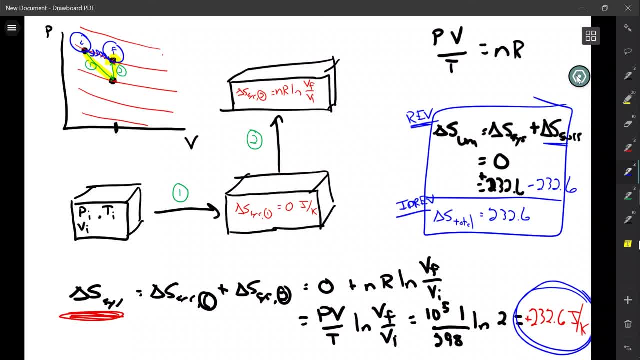 at the same time, you calculate the system increase by identifying a reversible pathway and evaluating the reversible heat interaction divided by temperature, all along that reversible pathway. and that's how we came up with 232.6 as the change in the system entropy. whether it was done reversibly or irreversibly, the change in the surroundings, entropy is the change in the. 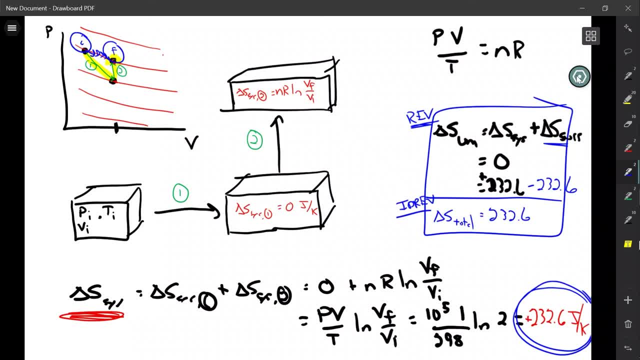 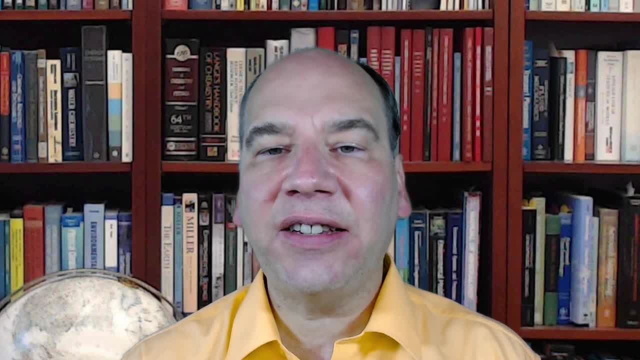 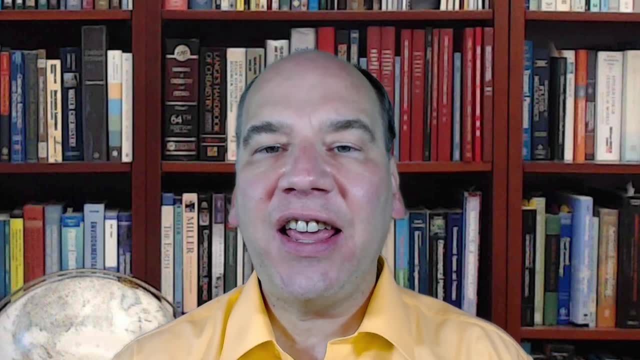 environmentün was zero in the case of being done irreversibly and minus 232.6 in the case of being done reversibly. so in review in in today's uh discussion, we did two things. the worst thing i did was we talked about qualitatively how there are changes in the world as we look about, and that seemed to. 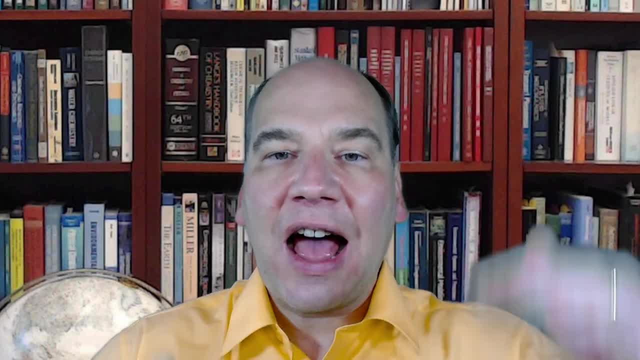 have a direction of time or a natural direction, a hot block next to cold block. one cools, the other warms. they come to the same temperature. if you have two blocks, the same temperature, you never observe that one warms and when you cool, one's gonna come up and the other one warms. then you'll never see more. 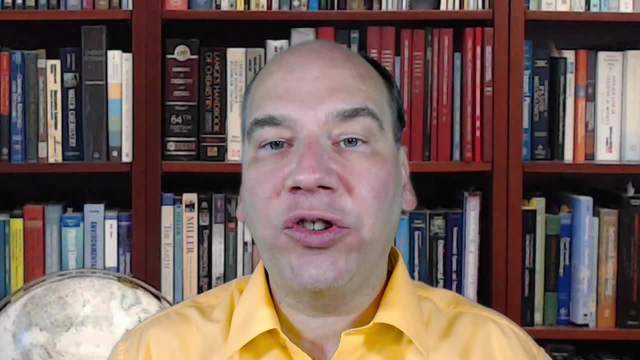 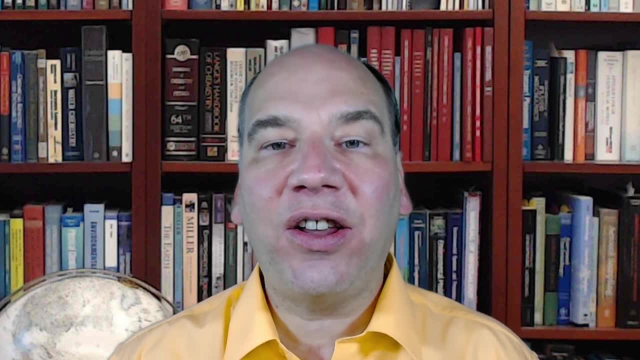 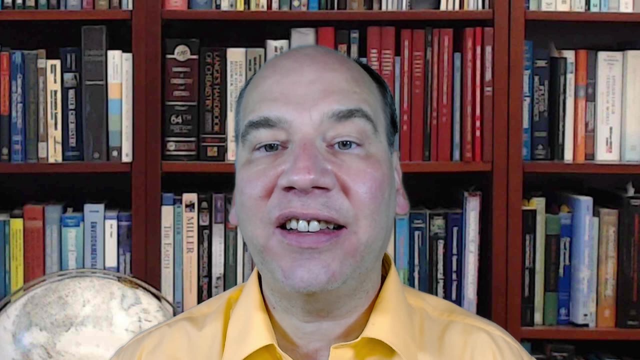 one cools. although that can, that uh conserves joules and would be fine by the first law, there's still something missing, and so we needed this idea of, of spontaneity. the second law comes into it and we developed that there's some mathematics. we defined a function, s, and we said ds, defined as the. 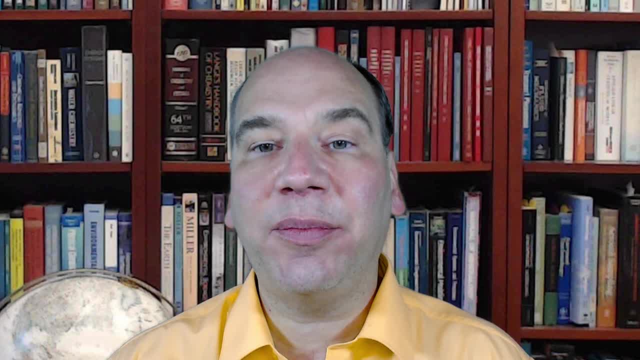 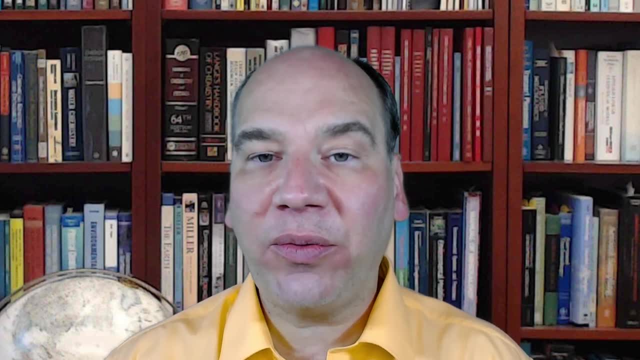 reversible heat interaction, ds, the system defined as the reversible heat interaction divided by temperature. we can calculate the change along a reversible pathway and delta s, the system plus delta s of the surrounding, which together are delta s total. that's equal to zero if we followed a reversible pathway. it's greater than zero and spontaneous if we followed an. 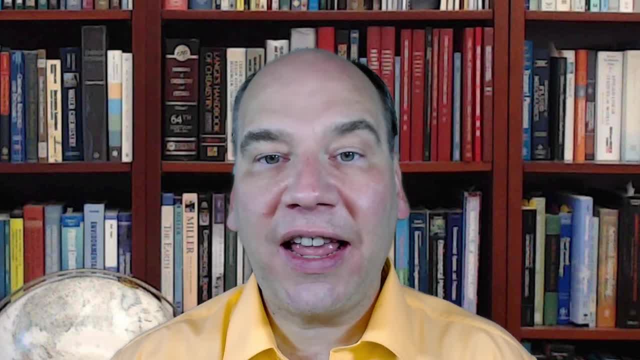 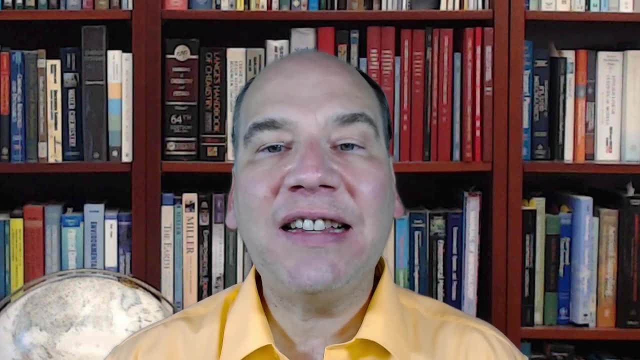 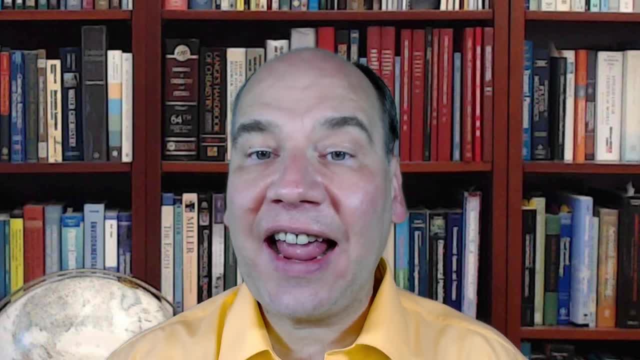 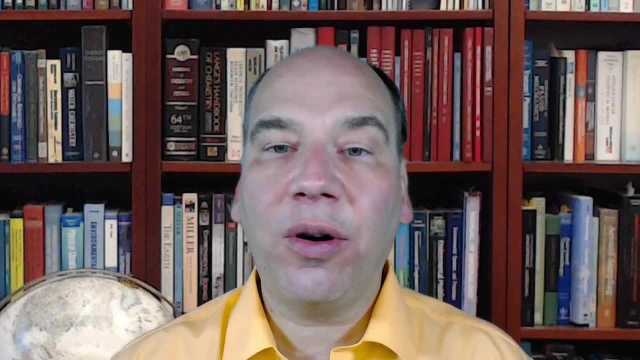 it's not a process. it's not a process. it does not mean fast, just means it can happen. maybe it happens like that, maybe the actual process is slow and maybe it takes a million years or a billion years. so spontaneous doesn't imply the time scale of the change: spontaneous.